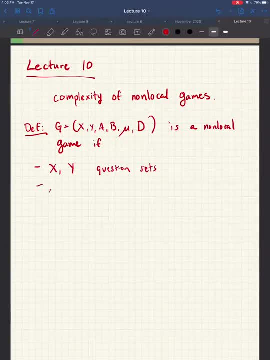 A and B are going to be answer sets. This mu is a distribution over questions from X and Y And this D it's what we call a decision predicate. So it sort of says when do the players win this game? So it's a function from questions and answers to zero or one. So if you want to know whether 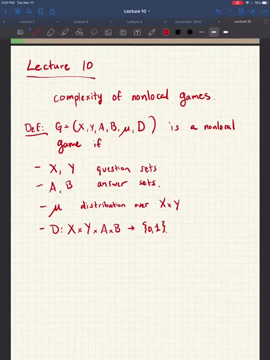 the players won this particular game. you just plug in the questions that they received and the answers that they reported, and this D function will tell you whether they won or not. So we call this the decision predicate, or just decision procedure. So that's what. 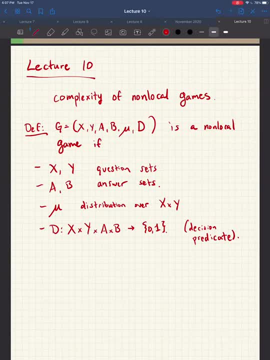 a non-local game is. And you know, suppose someone came up to you and said: here's my favorite non-local game. Here are the rules, Here are the question distribution: What is their maximum probability of success? Can you compute it for me, You know? is there an algorithm to do so? And 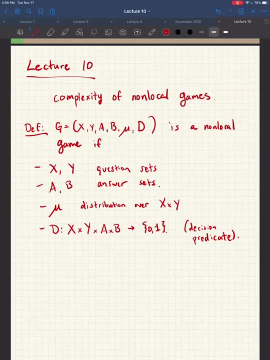 as we mentioned a couple of weeks ago. you know the it turns out, the eventual answer is: there actually is no algorithm to do this, And today we'll start to see, like, how do you prove such a thing? So you have a game and we'll we should say: what does it mean? 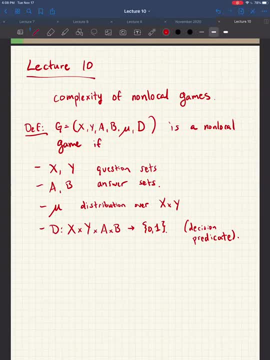 Like what? what does it mean to? how do you measure this optimal winning probability? So you have to talk about the types of strategies that the players are allowed to use. We're going to talk about quantum strategies, cause that's what we're interested in, But there's 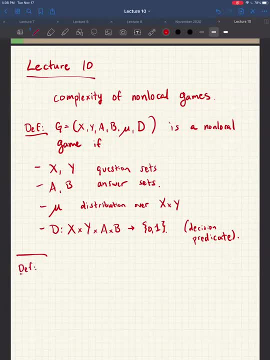 there's different kinds, So so here. Okay, Here's a definition of a quantum strategy. So I'll say a, a finite dimensional strategy for a non-local game, G it's going to be, you get to pick. okay, This is a, this is a quantum strategy for a non-local game. right, And now you're. 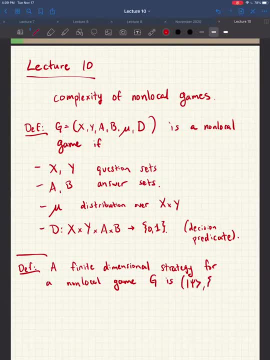 going to see how a random game works. This is going to be the, the, the. I call it the linear momentum strategy. Okay, Now you'll notice, here is the, the, the, the non-local dynamic strategy. This is going. 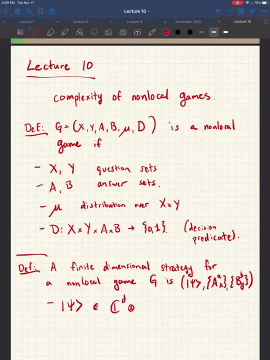 to allow you to see the linear momentum strategy for for a non-local game of for a non-local game. but I can't tell you exactly what I'm talking about here, because it's sort of a much more complicated logic than this. Okay, 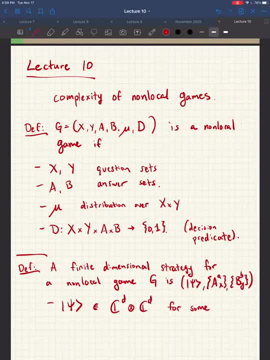 So so here we're looking at the, the, the, the non-local game, The state of a quantum for some finite D, and then these measurements they're going to be, you know, some choice of D dimensional positive operators. that's onto identity, yada, yada yada. 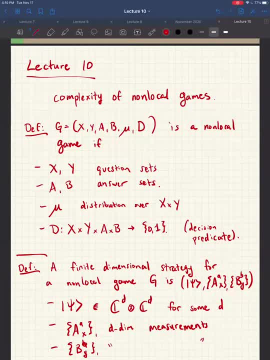 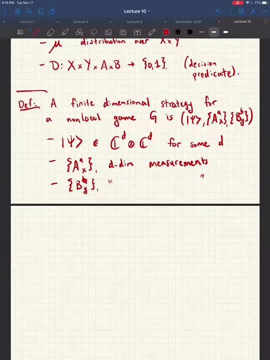 Okay, So if you, if Alice and Bob, decide to use such a strategy, what is their success probability? So so I'll say that it's going to be omega of this game G and you fix this particular strategy. So what is it? 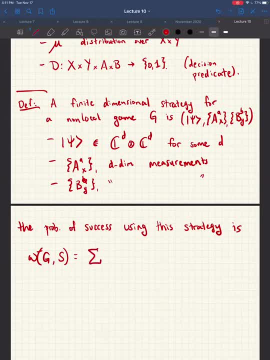 Well, you say I'm going to choose the questions X and Y at random from this question distribution And then I'm going to sum over all possible answers that they could produce that would lead them to win the game. So you say I only care about the A's and B's. 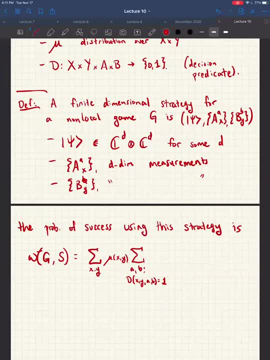 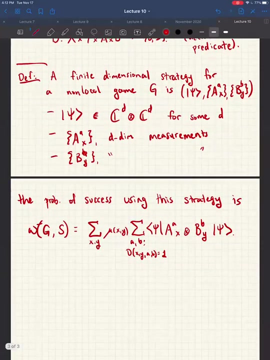 that have them win. And then you have to put in the probability that they, when they perform their measurements, they actually generate this particular A and B. So that's given by this expectation value. Okay, So hopefully that should make sense. Now we can define the quantum value. 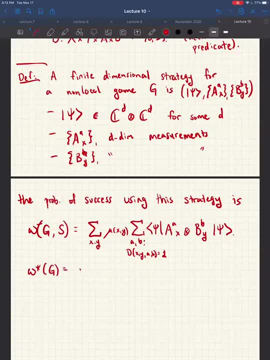 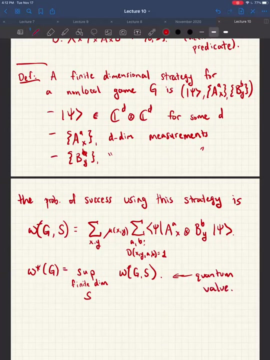 to be this omega star of G, And we've seen this before, right this before. This is going to be the supremum over all finite dimensional strategies S of their success probability, given that strategy. So we call this the quantum value of the game. 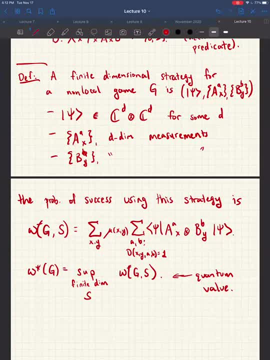 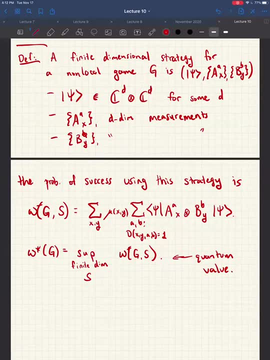 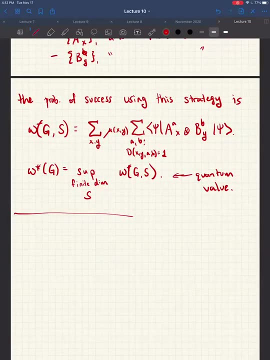 This is how well they can do if they use a finite number of qubits in their strategy. So the complexity question was the computational problem is: given G, can you estimate omega star G? say plus or minus some small constant like 10%. 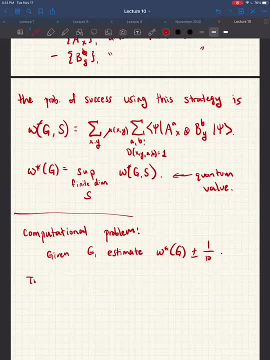 Can you come up with an algorithm to do that? It turns out no. So I mentioned last time that. okay, so that itself is already pretty interesting, But you know there's more to be said, because it's actually connected to. 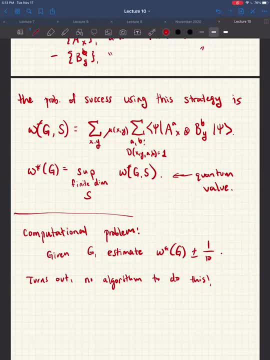 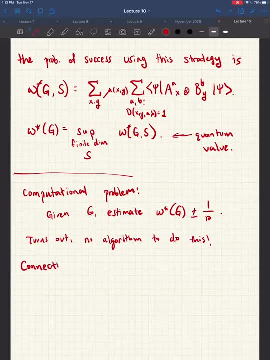 seemingly unrelated questions in other areas. So the last time we left off with you know their connections to, say, mathematical physics, And there the question is: Can you remind us if that's a proven result, the fact that there's no algorithm? 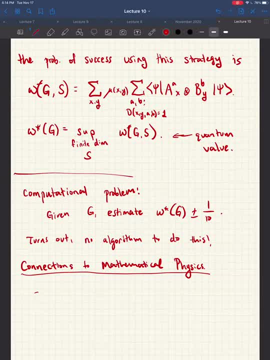 Yes, So this is a proven result And we're going to see at least a high level of what goes on into this proof. Yeah, So I think last time someone- I forget who asked, but someone asked: is it that we don't know of an algorithm or we know that there is no algorithm? 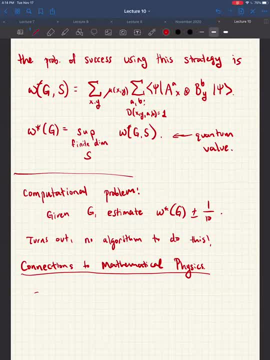 And it's the second thing, We know for sure that there cannot be an algorithm, Okay, So. so what are these? these other connections? And you know, last time we had this very interesting, you know, discussion about finite dimensional versus infinite dimensional. 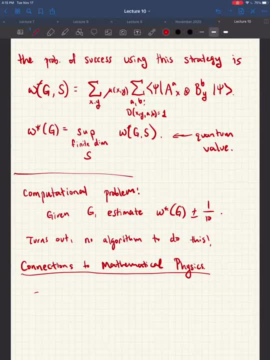 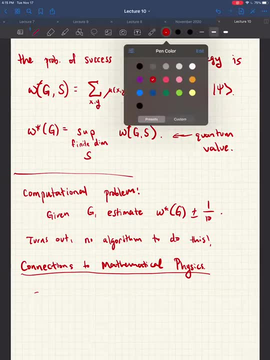 entanglement, and you know whether nature can be described, you know, can be described using finite dimensions only, or is it inherently infinite dimensional? So so this complexity question gets into that. So so here the question is: is 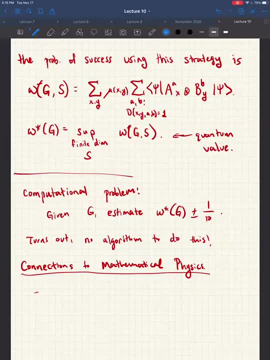 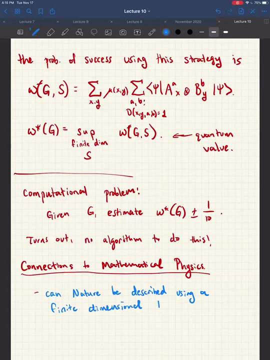 you know at the start, not about complexity theory or anything, it's just saying: can nature be described using a finite dimensional theory or is it inherently infinite dimensional Right? And you know, and I guess if you take like a standard quantum mechanics class, 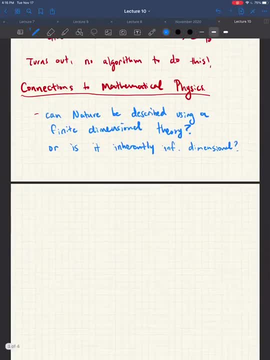 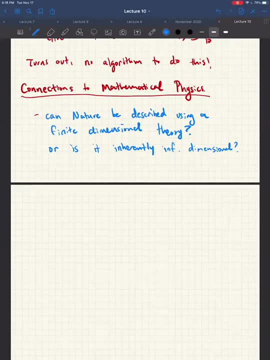 or something. a lot of things are presented naturally in in, in infinite dimensions, right? Like the Hamiltonian describing a hydrogen atom, it acts on an infinite dimensional space, right, And then there's the but, you know, the Hamiltonian, the Hamiltonian. the Hamiltonian is an infinite dimensional space. 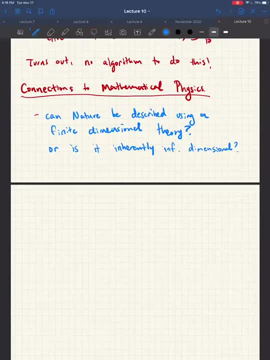 Right, And so you, you can just write what you want and you get the results. And so you might think, actually, maybe it's inherent. On the other hand, like if you're coming at things from like the quantum information theory point of view, 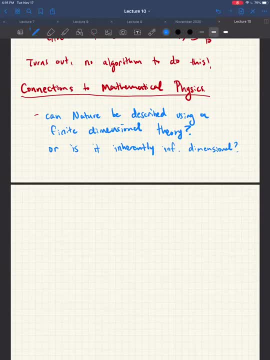 everything's taught in terms of finite dimensional Hilbert spaces, right? So you know what's the more appropriate model of nature? I guess this you know, this can get like quite philosophical and maybe it's you know, I don't think you know. 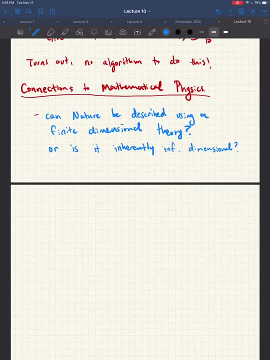 we're anywhere close to resolving this, but there's actually a really precise way in which we can get some angle on this question and actually come up with a precise mathematical answer to it. So we'll instantiate this question by asking: you know, in the context of non-local games? 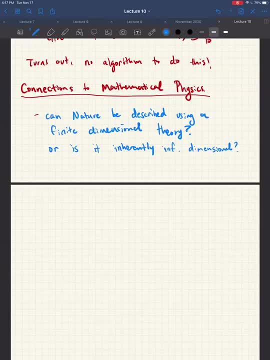 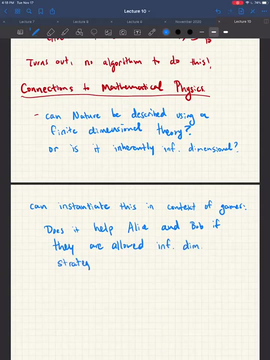 does it make a difference if Alice and Bob are allowed to use infinite dimensional quantum states and quantum strategies, Right? does this infinite dimensionality offer them any advantage? And so this is a very well-defined question, and you can hope to answer it All right. so that's the question we'll look at. 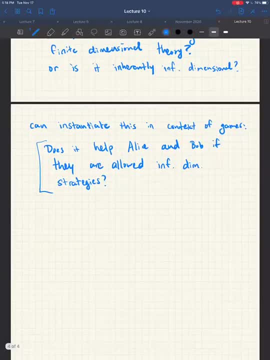 And I should define like: well, how do we model infinite dimensional strategies? And last time we talked about a couple of models. The most straightforward generalization to infinite dimensions would be: well, instead of this quantum state, psi, being in CD, tensor CD. 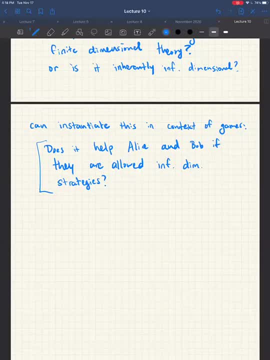 why don't I let it be in H tensor H for some infinite dimensional H? I mean, this is fine. You know you can talk about such things, but it turns out that this model can actually. it doesn't give you any additional. 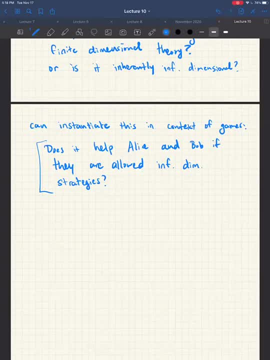 you know, additional power on top of finite dimensional strategies, at least in terms of non-local games. You know, whatever infinite dimensional strategy they use in this form, they can approximate it arbitrarily well using a finite dimensional strategy. Okay, so this generalization is maybe not so interesting. 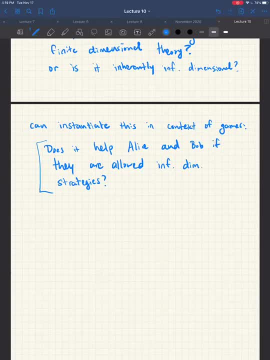 But there's another generalization called the commuting operator model, which you can say more things about. So this is how we model infinite dimensional strategies. So you choose a state, you have measurement operators, as usual. So this state, all you say is that it's just a vector. 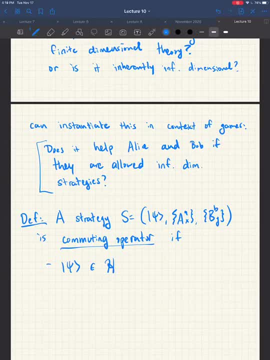 in some Hilbert space. okay, This Hilbert space doesn't necessarily have any tensor product structure. It can be finite dimensional, it can be infinite dimensional. These operators, they're measurement operators, They all act on the same space, But in order to make things like in the setting. 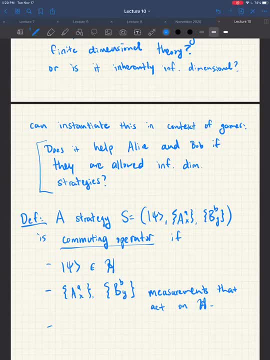 of non-local games, we have this constraint that Alice and Bob can't talk to each other, right Like they cannot. they get an input, they get a question and they don't know what the other person's question is. So you need to install that into the definition somehow. 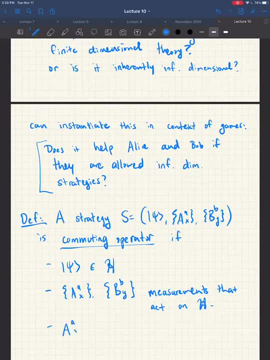 And that's from the constraint that they're- that measurement operators commute And what that means is Alice and Bob, they're gonna measure the state psi and they're measuring in the same space. But since their operators commute, it doesn't matter which order they measure. 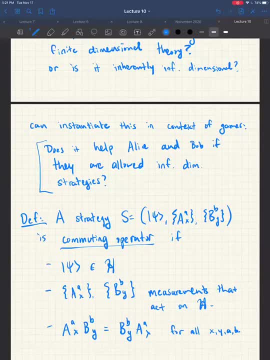 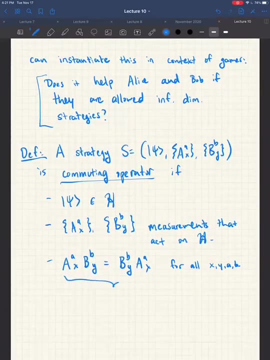 Like Alice can measure first, Bob can measure first The statistics of the, their outcomes will always be the same, And what that means is they can't do anything to like send the signal to the other person. So then you know, the parameters are gonna be all the same. 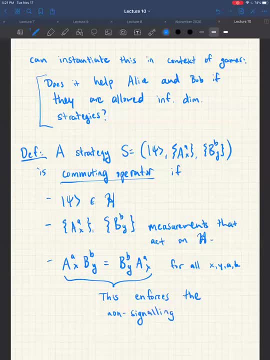 So we're gonna have to try and do this in a different way. So I think it's really important that we make sure that we're all getting the best and the best performance we can give them, And I think that's a big asset to really essentially doing the math. 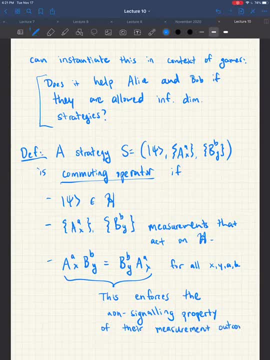 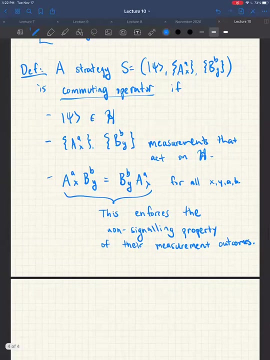 and figuring out how to get them to move in the right direction If the operator has to come to a different location, like say: Okay, any questions about the definition of commuting operator strategy. So you know, if they decide to use this kind of strategy, then how do you measure their 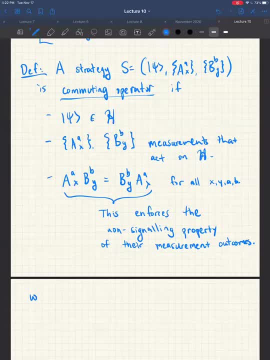 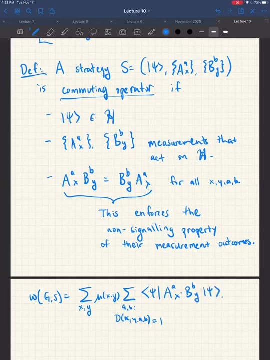 success? Well, it's largely the same. You just omit the tensor product signs, because there's no such thing as a tensor product. We just have this same expression. This is the probability that they win. So here, instead of tensoring the operators together, you just multiply. 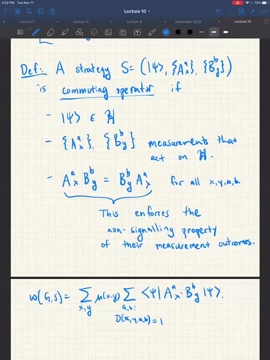 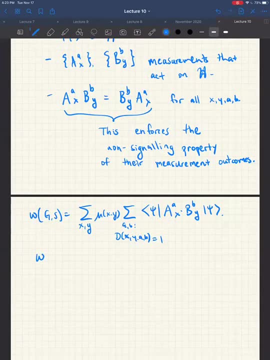 But again, you know, the order in which you multiply them doesn't matter. And so, if we allow ourselves to maximize over these kinds of more general strategies, we call this the commuting operator value of a game, And so this is the supremum over commuting operator s of omega g, comma s. 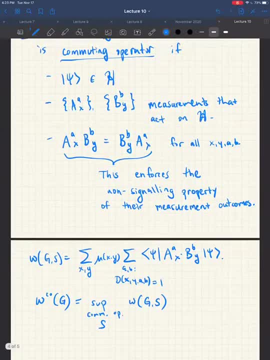 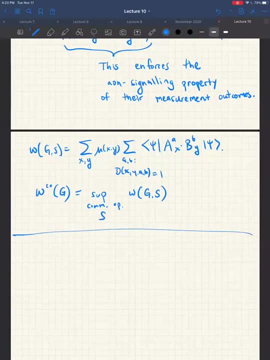 So this is a different kind of value, and one easy thing to see is that the finite dimensional value, or this quantum value that we defined before, is always, at most, the commuting operator value. All right, All right, And this is because the commuting operator strategies are just a strict generalization. 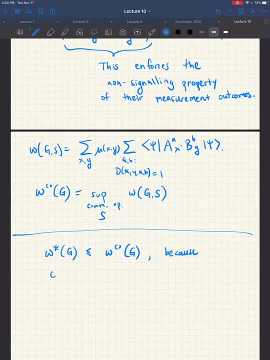 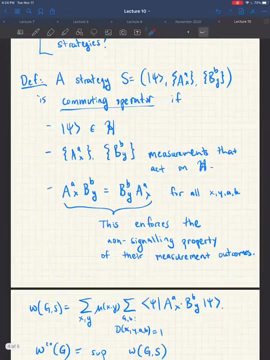 of finite dimensional ones, Right Like because you could have imagined that you know if you were to do this, if you were to do this, you could have imagined that you know this. Hilbert space h here was actually a tensor product of two spaces: Alice's space, tensor Bob's space. 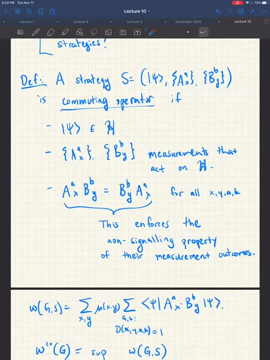 And then their operators is. you know, if you look at it closely it really looks like you know some operator on Alice's side, tensor, the identity. And then for Bob's measurements, it's identity on Alice's side tensor, some operator on Bob's. 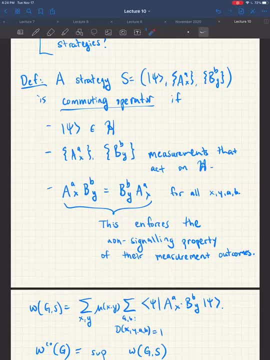 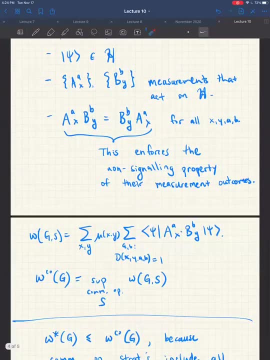 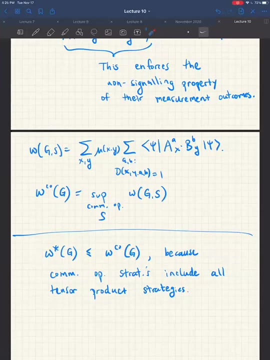 side Right. So basically, Alice's and Bob's operators will commute. What is W star, Omega star here? Yeah, Omega star, Yeah, That's the finite dimensional value, or the quantum value. It's their maximum success probability when they only restrict to finite dimensional strategies. 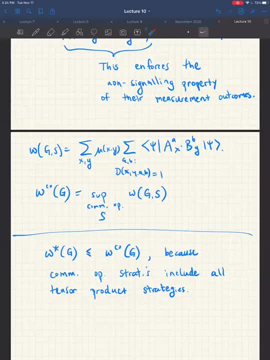 But that's the quantum one, right? Yeah, I guess it's maybe a little ambiguous when I say quantum, because you know you could also say that the commuting operators thing is also quantum. I guess it's just like a. it's just a naming that stuck. 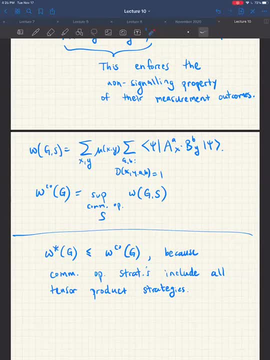 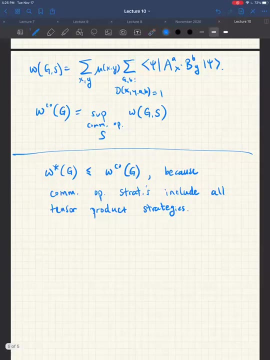 Yeah, Actually, maybe just to make things clear, we'll just say finite dimensional value versus the commuting operator value, just to make things perfectly clear. Okay, Okay, Okay, So, so we know this, this fact, and this holds for any game you walk up with. 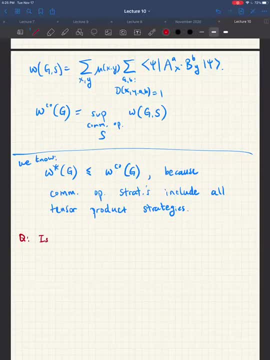 But the more interesting question is: is there a game g such that there's actually a difference between these two values, Between the finite dimensional value and the commuting operator value, Right? So if? if that were the case, then it would mean that in this game g, if Alice and Bob 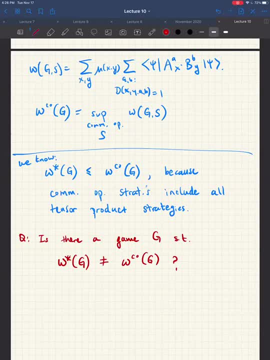 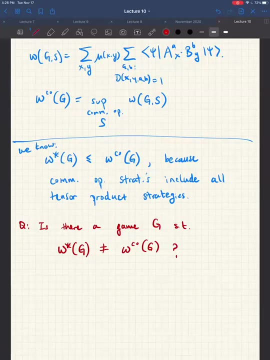 decided to use this more general commuting operator strategy, they would be able to achieve a higher winning probability, So it actually benefits them. Um, and and actually, uh, in that case, Um, it's, you know, not only is this, you know, better strategy- a commuting operator. 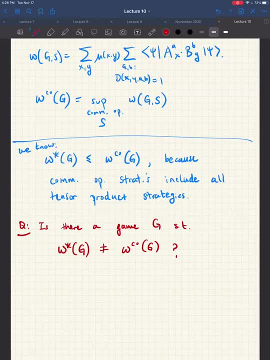 strategy, it has to be infinite dimensional, Um, and the reason that's the case is, uh, if you restrict yourselves to finite dimensions, um, then, uh, well, I, I guess it's, it's by, um, uh, oh, right. 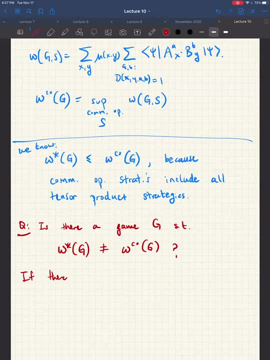 So so you know. the point is, if you're in the commuting operator, Um, realm right, There's no notion of tensor product. but you say that the Hilbert space is finite dimensional, Then in fact it turns out that you can, um, actually find a tensor product decomposition. 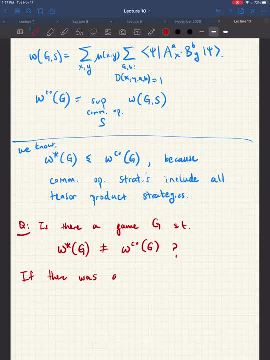 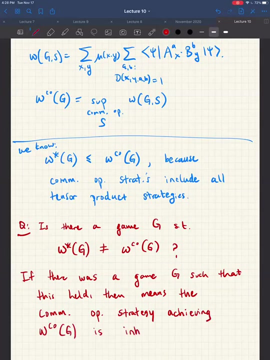 of your space. Okay, Okay, So, uh, there's still some logic to this. So you guys see, now let me just make this a little bit easier. Let me, let me just make this a little bit easier, Okay. 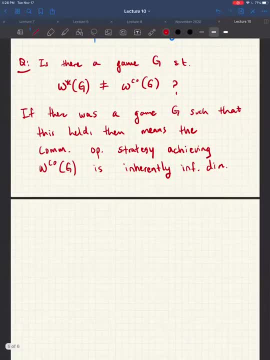 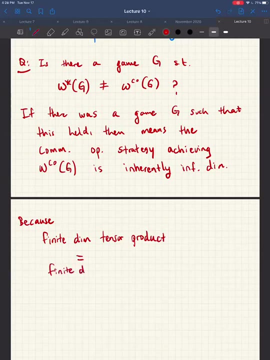 So if you look at: Oh, let's see. So you know I won't show this here like this, this is some, I guess some result in functional analysis. but it's true, If you're in finite dimensions, there's no distinction between 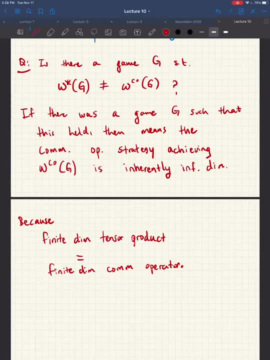 tensor, product spaces and commuting operators strategies. So if there is a difference- you know that's this question- then it must be because there's an inherent advantage or inherent difference between finite and infinite dimensions. So one of the things we mentioned last time is that, you know, suppose there was such a 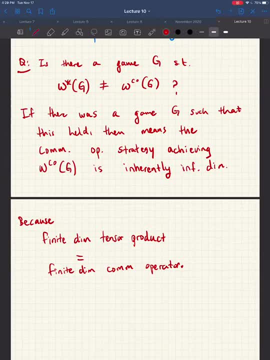 separating game, right, a game where finite dimensional and commuting operator value were different, then this game would be, in principle, some kind of experimental test of infinite dimensionality. right, Like you know? imagine you're playing this game between with your lab equipment and then you know, you see that the winning probability is. 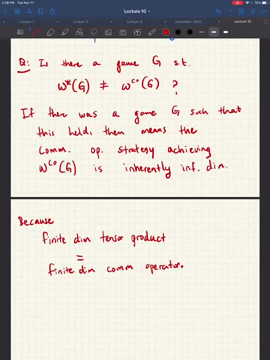 tending closer to this omega co-value rather than the omega star value, Then that suggests that whatever nature is doing, you know, inside your lab equipment, it cannot be described using a finite dimensional strategy. Okay, so this question is known as Sirilson's problem, right, This is named after the same. 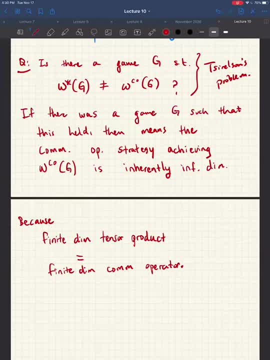 Sirilson, who came up with the question right. So if you're in a finite dimensional strategy, you know you can't do better than this 85% number And you know it's not an easy question, Like all the non-local games that we saw so far, you know CHSH, Magic Square and so on. 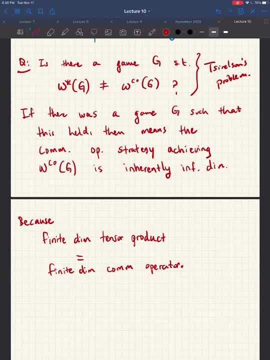 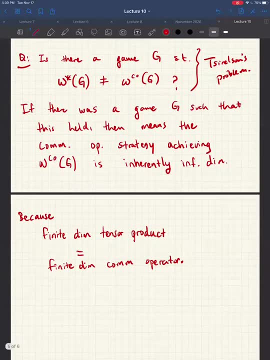 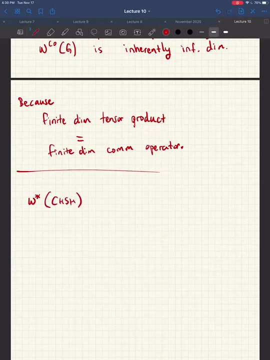 none of these exhibit a separation between the finite dimensional and infinite dimensional values. So, you know, the omega star of this CHSH right which we saw was, you know, this 85.4% value. it's the same as the commuting operator value. You know same thing with Magic Square. 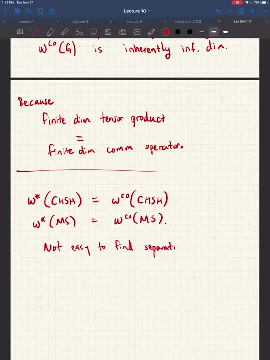 So you know you can't do better than this. Okay, so that's the mathematical physics question. Here's where it connects back to this complexity. right, I mentioned that, this question of: is there an algorithm to estimate the value, this omega star value of a game? somehow connected to this finite versus infinite. So I'm going to go back to the question of: is there an algorithm to estimate the value, this omega star value, of a game somehow connected to this finite versus infinite? Okay, so that's the mathematical physics question. 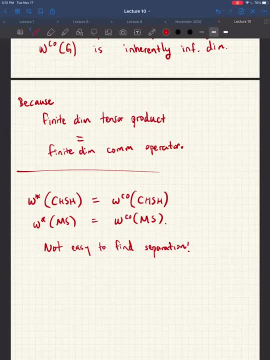 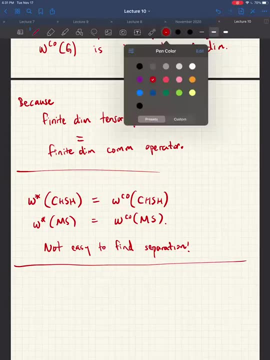 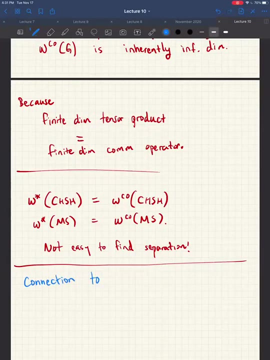 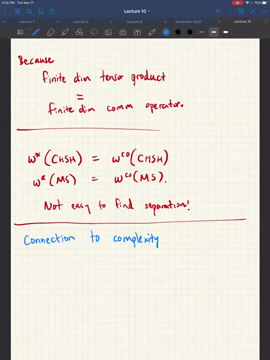 So I'm going to go back to the question of: is there an algorithm to estimate the value, this omega, star value of a game, infinite dimensions? it comes through the following: Here's a different column. So if it were the case, you know, imagine that we were in a world where, if no matter what game you came up with, 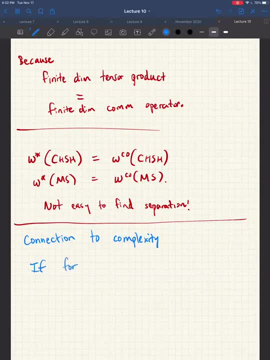 there was no difference between these two values. You know, not only would it say that, okay, infinite dimensional strategies don't help you at all, this would have the interesting consequence of giving us an algorithm for estimating the quantum value of a game. 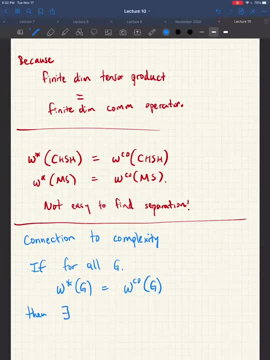 So if it were the case, you know, imagine that we were in a world where, if no matter what game you came up with, this would have the interesting consequence of giving us an algorithm for estimating the quantum value of a game, Right, which is the thing we were wondering about in the beginning. 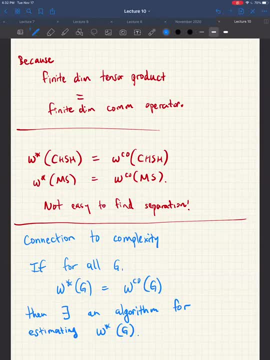 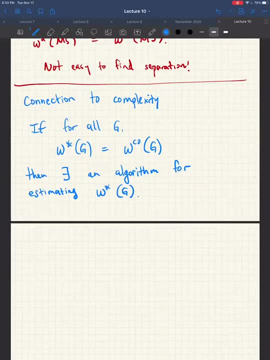 So you know how does this work? Well, it's because we can actually combine two different semi-algorithms. So one semi-algorithm- and I'll explain what that means in a minute- will approximate this finite dimensional value from below. 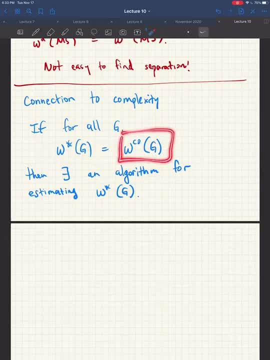 And the other semi-algorithm will approximate this commuting operator value from above, And since, if we're assuming that they're always the same, then these two semi-algorithms will actually converge to the correct quantum value. So the first semi-algorithm- 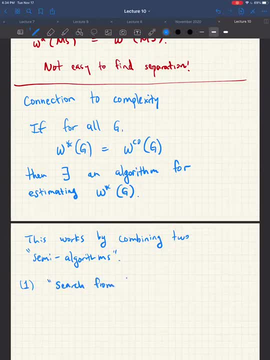 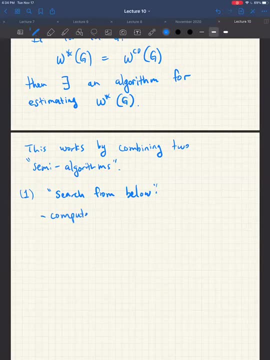 let's call it a search from below. So what does it do? Well, it's an algorithm that it just computes the sequence, this infinite sequence of numbers: alpha, one, alpha, two, dot, dot, dot- And it's just gonna keep computing them. 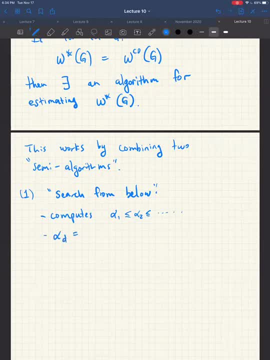 And what's an alpha? So alpha D is going to be the best winning probability to get the same result. So we're fixing some non-local game G here. We fix it ahead of time using a D dimensional strategy. So if you remember from our discussion from last time, 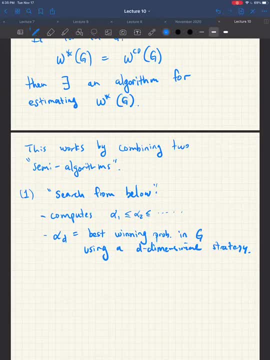 if you fix the dimension of the strategy you're considering, then this alpha D, you can actually approximate it right Like cause, you can discretize the sum right, the space of the strategy, and it turns out that there's only like a finite number. 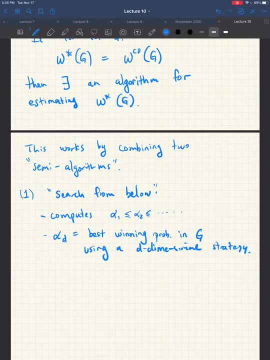 of possibilities you need to consider. So you can, you know, in the worst case, numerate over all of them and just pick the best strategy. So this alpha D, it's computable in some finite amount of time. So for any given D you can just compute it. 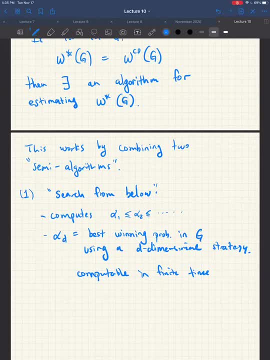 Clearly these alphas form a non-decreasing sequence, right Like if you increase the dimension of strategy that you allow the players, they can't do any worse. The other thing we know about this alpha D is that in the limit, as D goes to infinity. 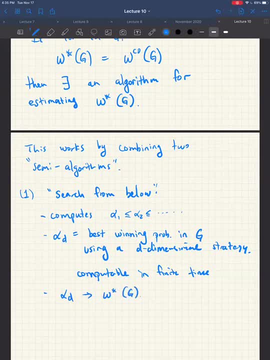 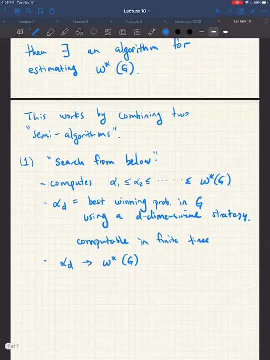 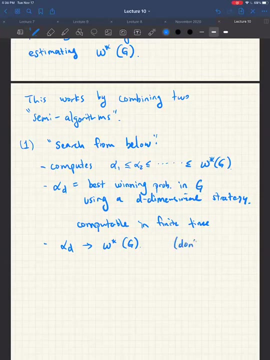 it will approach this omega star value, right? So all of these are lower bounds on omega star and they will eventually converge there. You know, the issue is that we just don't know how fast. Right, and that's a major problem because you know. 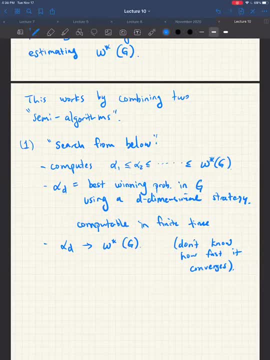 you're running this algorithm and you just don't know when to stop the algorithm, because you don't know if you're any closer to you know if you're at all close to the true answer. So that's why I call it a semi algorithm. 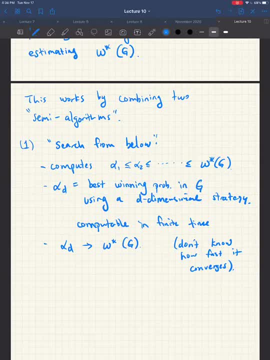 Like you can just run it forever and it you know, we just know that in the limit it gets closer and closer to the correct answer. Right, so hopefully this rings a bell. The other semi algorithm is what I'll call search from above. 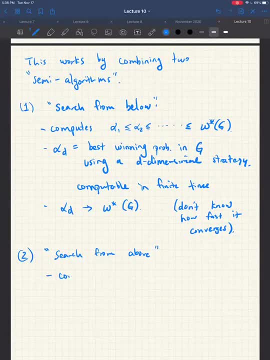 And it also computes an infinite sequence of numbers. So it computes beta one, beta two, so on. But this time these numbers are not going to be the same. these numbers are, you know, they're not increasing, They're slowly getting smaller and smaller. 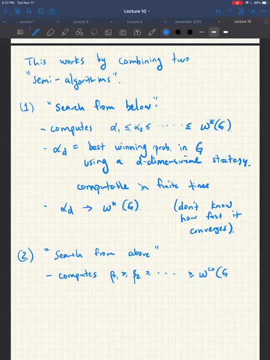 They're all going to be upper bounds on this commuting operator value. Okay, What is this beta D? Well, it gets a little more technical to state, but it's some quantity that's computed from some convex optimization problem, And you know. the point is that they're all just guaranteed. 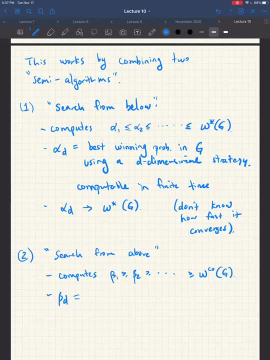 to be upper bounds on this commuting operator value. You know, if you're really curious what it is. it's you know the best, or this is this. It's some solution to an SDP relaxation. Yes, exactly, It's yeah. so you know, if you know what, what an SDP? 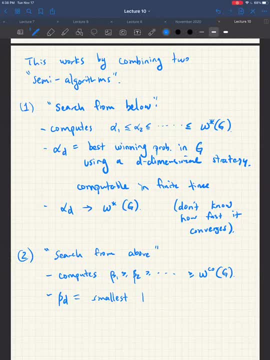 what an SDP relaxation is, then that's what it is. It's the smallest number, such that beta D minus your target value, this omega co. the fact that this is non-negative is certifiable using degree D. sum of squares polynomials. 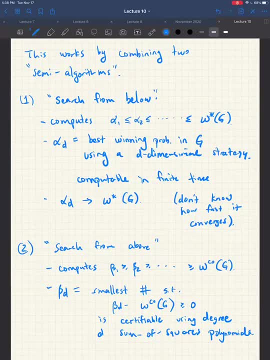 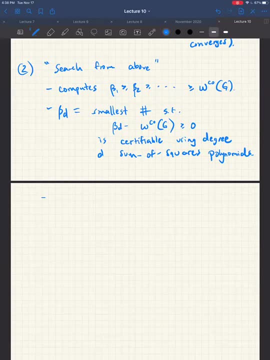 Okay, whatever this is, The important thing is that if you plug in, you know you fix a D, you can write a program to compute this number. In fact, you know there are even packages you can download online that will do this sort of thing. 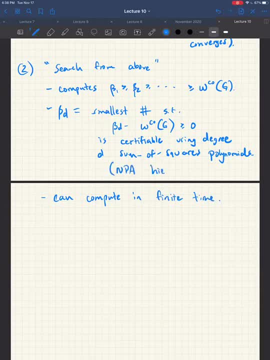 This is What did you say. they were called Yeah. okay, Which thing was called Yeah? the beta Ds are the solution. I don't know if someone said some technical term that I was gonna Google, but I don't remember what it was. 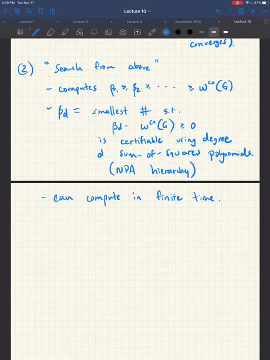 Like, what are these beta Ds? Oh well, it's sort of what I wrote. It's like the smallest. it's basically the solution to a semi-definite program And a specific semi-definite program and if you wanted to Google it, 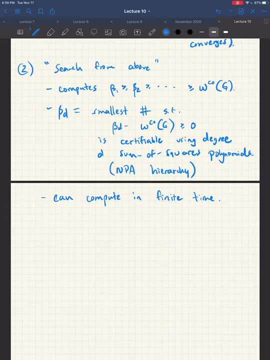 you can look up this thing called the NPA hierarchy And there is software that people have written that actually implement this convex program, You know, but for this discussion we don't necessarily care exactly what the definition is, So you can compute this in finite time. 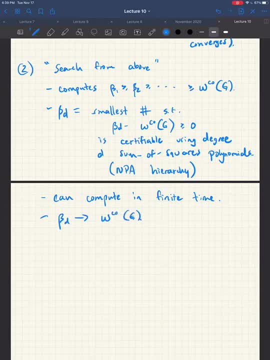 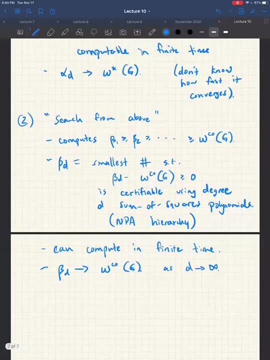 and beta D will converge to omega co as D goes to infinity Right. so, and again, we just don't know how fast this is. We don't even know how fast it converges. So you probably see where this is going. 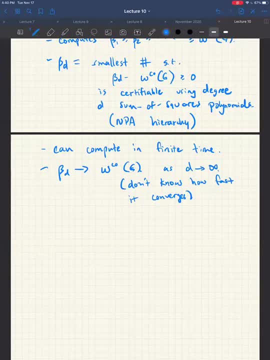 Right, like we can put these two things together. No, imagine that we have this. someone hands you a non local game. it has some true quantum value that we're trying to estimate And we're assuming that. suppose it's the same. 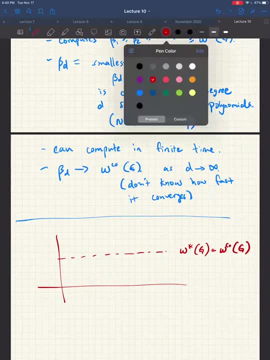 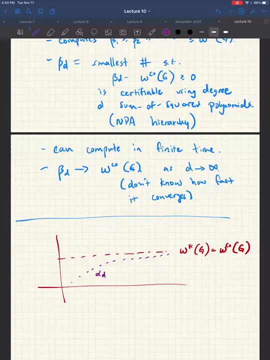 as its commuting operator value And we can compute from both sides these alpha Ds. So D is going to infinity. We can also compute these beta Ds, Since they're both guaranteed to converge. we know, at some point they're going to get. 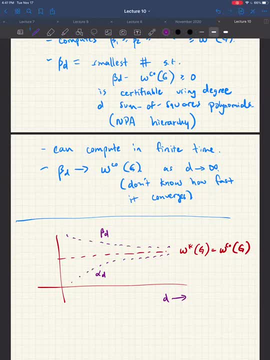 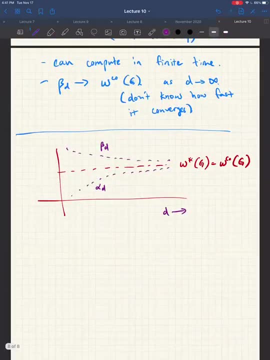 within epsilon of each other, at which case your algorithm knows. aha, I've homed in on the correct value. So you said before that we know this doesn't exist, right? The estimating algorithm In general: yeah, Sorry, one sec. 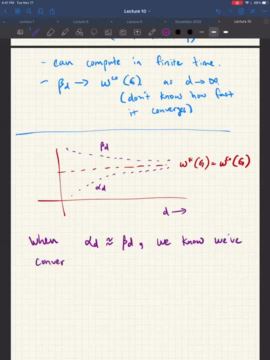 I'm sorry. So if this happens, then we know we've converged to this value, and then that's it. You've estimated this omega star right, So I've presented you an algorithm that works, if under this assumption that these two values are the same. 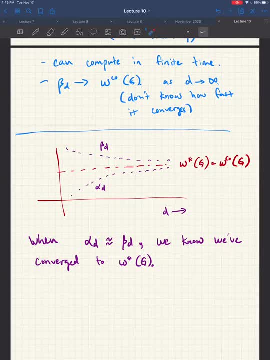 So you know, you've got some kind of a hypothesis about what's gonna happen if this algorithm does table for all G. So in other words, then an algorithm to calculate the winning probability exists if, and only if, for all G these numbers are the same. 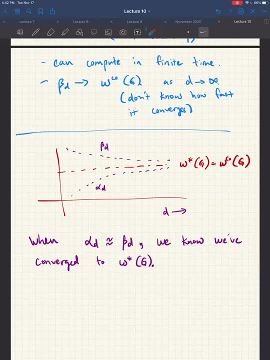 And the algorithm doesn't exist, even if you're applying it when they are the same, unless all G obey this property. oh, not that strong um. so so this is a fact. if they are the same, then this algorithm that i just described, like this algorithm you can even code up today. it will work. 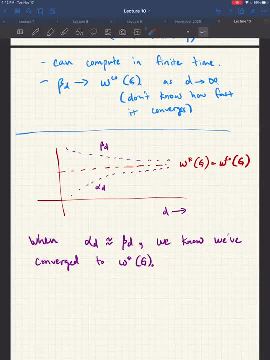 i mean it'll take forever, um, but it will work. um, uh, but uh. if for any game for which they are not the same, then then the, the, your algorithm will just spin its wheels and these two sequences will, will not converge. and you're just wondering: wait is it? is it going to converge at some point, or? 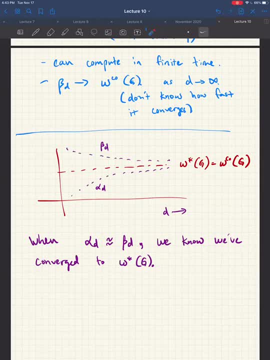 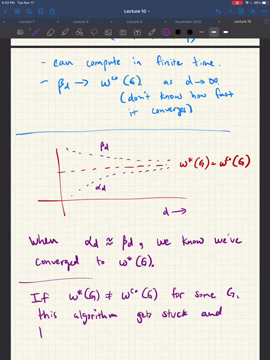 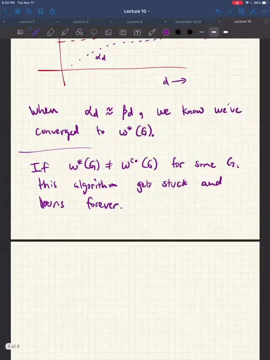 are they really different? um, right, which is what lands it in the uncomputable class? yeah, exactly so. so so you, you, um okay, so, uh, right, so so really now, um, this question of, so we've we've tied the two questions um whether infinite dimensional strategies help or not is directly tied to whether there's an algorithm to 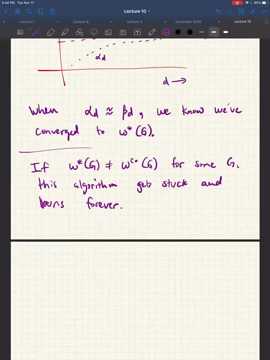 approximating this, um um this game, you know maximum success probability, right, um so? so that's one connection. uh, any other questions about this link? yeah, um, sorry, can you hear me? it's a little bit glitchy on my end. yeah, can hear you. uh, am i jumping ahead of it? uh, since you said, 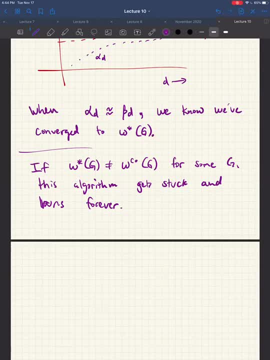 yeah, can hear you. am i jumping ahead of it? uh, since you said me there is no algorithm that can do this, that's been proven. that there's no algorithm that can do this, and now there is an algorithm that if they're equal, then they're not equal. is that where we're going? yeah, yep, exactly, um right, so so? that that is the correct uh implication. um, so we're going to show that there is no algorithm for estimating omega star. so, in particular, the algorithm i just described cannot work for all games. g which tells you that you're wrong is that it's not fair to just read the game. you're wrong. but know that if patients cannot work for a certainbulk and are highly poorly able to access, this might even give you problems, which you need to do. so we mention this by saying: just know, here there's a holding. thank. 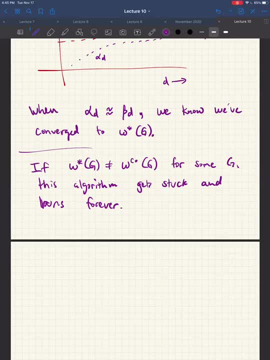 game out there don't know what, but some game where there is this difference. Wouldn't that by itself indicate that our earlier question about whether we need infinite dimensional spaces to model the world, wouldn't that say, yes, we do. I guess it would. I would view it as it still leaves open the possibility that 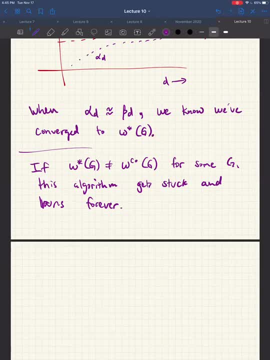 you need infinite dimensional spaces, because you know this. if there is a separating game, it's not clear at all that this game is experimentally realizable in our universe. It just says that, at least mathematically, it's not ruled out. 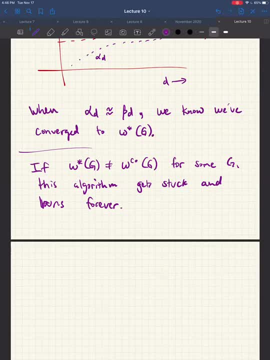 So this is the solution to Sirotson's problem, but we just don't, like we haven't found an actual game that does it, but like we know the answer. So yeah, we know the answer. In fact, we do know of the game, like 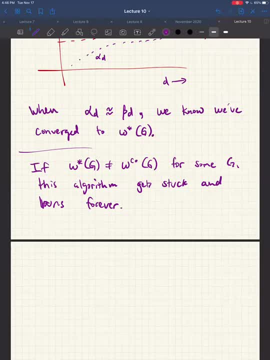 we can write down a description of the game, but it's still very mysterious, like the description of the game is very opaque, Like it doesn't tell us anything about what this so this game we know for sure, like I can write it down and this you know, I know this game has infinite dimensions. help. 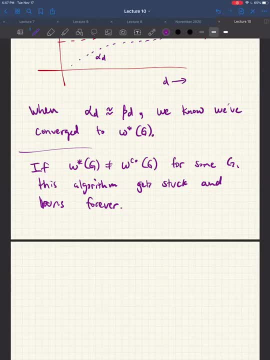 you know you can do better using infinite dimensional strategies, but we don't. we have no idea what this infinite dimensional strategy looks like. We just know there's a gap, Yeah, But I'll see more about this later. So it's a game that then no one has ever won. 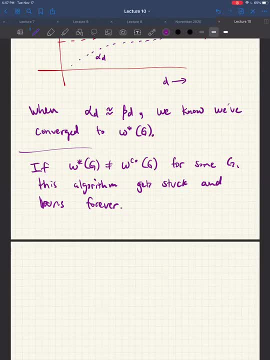 At least no one has ever won with the mathematically allowed maximum probability. You know what am I even saying? No one's ever played this game Like. it's only been written down like theoretically Right. Is there any notion of playability in a non-local game? 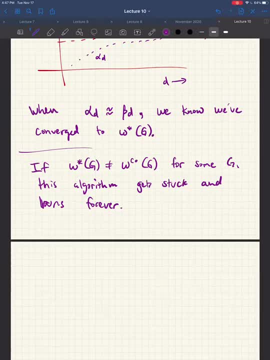 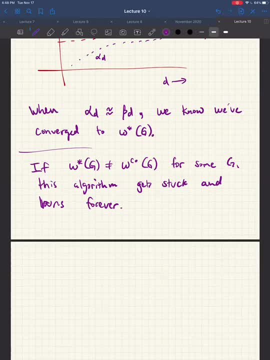 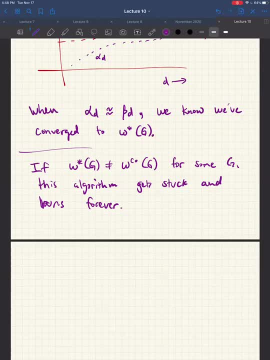 do some faster than light speed travel or to manipulate you know. three qubits each maximally entangled with each other. you would have an unplayable game. Is there something in the lexicon of these games that already forbids other? 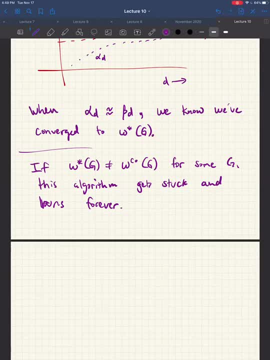 I see what you're asking. I'll say this: I guess this game it's formulated within the mathematical framework of quantum field theory, So okay, well, there's a couple of things Like. one is that apparently there's still no well-defined 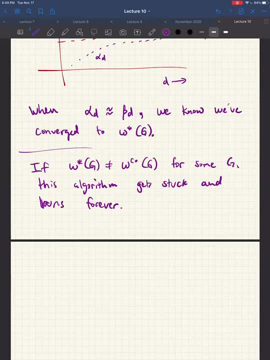 mathematical, like rigorously formalized mathematical framework for quantum field theory. This is actually. people are trying to figure this out, but at least people agree on some basic axioms And this game is compatible with those axioms. So as far as we can tell, 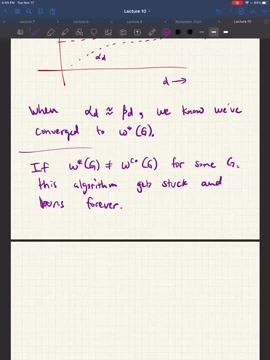 it's Yeah, Yeah, Yeah, Yeah, Yeah. It's compatible with what we believe is allowable by quantum field theory. But the question is whether you know all these, Whether you need more than just these bare axioms that people have listed. 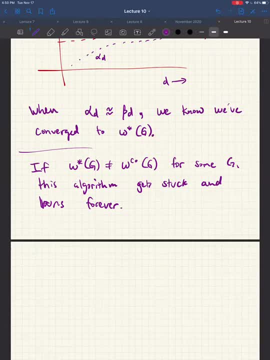 Yeah, So Where am I going with this? Yeah, I don't know. Hopefully that kind of answers your question. maybe You know so just concretely, like you're not allowed, You know it won't allow you to. 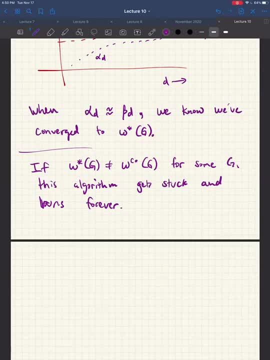 like you know, manipulate three qubits that are massively entangled, because that violates the axioms of basic quantum mechanics. So that's not something that happens here. All right, That does help. Okay, So this is, you know, a connection to quantum field theory. So you know, this is you know. 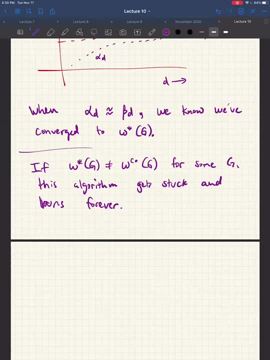 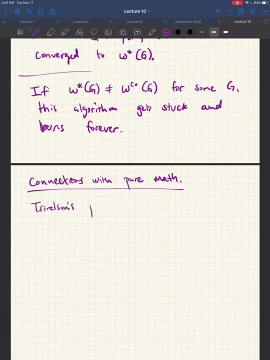 a connection with finite versus infinite, And now let me just quickly mention this connection with this area of pure math. So the Searleson's problem turns out to be equivalent And people only discovered this like 10 years ago. 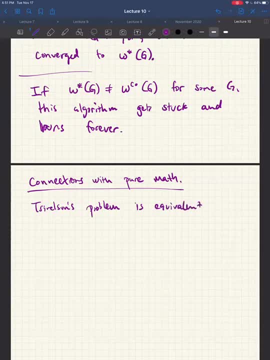 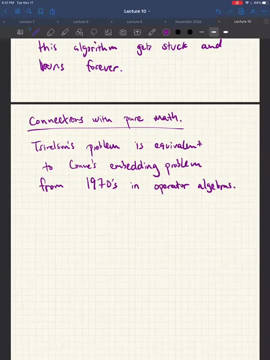 Yeah, It's equivalent to something known as this con-embedding problem. This is a problem that was formulated in the 1970s in this area of functional analysis called operator algebras. Okay, You know, I know basically nothing about operator algebras, but at least I can try to. 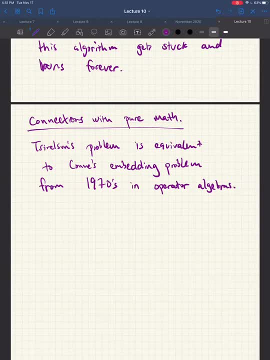 convey what I think is a sort of a cartoon picture of what this con-embedding problem is about Like. if you, you know, look up the Wikipedia article on this embedding problem, you know it's just like a lot of words that you know, at least I've never heard of. 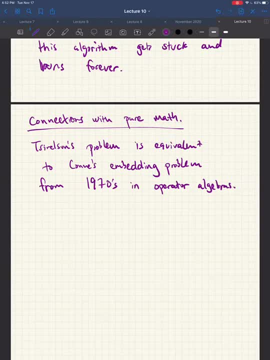 But let me You know, I think it's a good question. Yeah, Yeah, Yeah. Yeah, I think I have some cartoon explanation of it. So it's about something called von Neumann algebras. What's a von Neumann algebra? 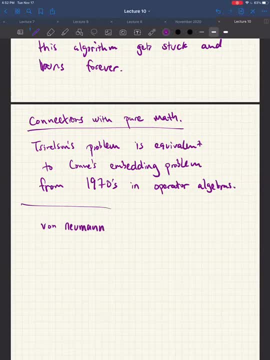 It's basically some abstract set of operators acting on a Hilbert space- Okay, So it's a set of operators acting on some Hilbert space H- Okay, Okay. So generally, people really like the Hs that are infinite dimensional. 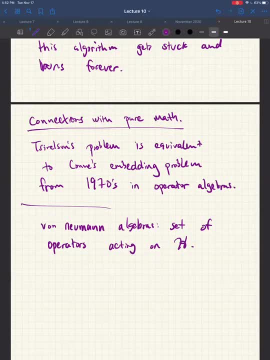 Those are the most exciting ones for the mathematicians Also, by the way, if someone in this you know in the audience, like you've taken a class you know, like, feel free to jump in and save me. 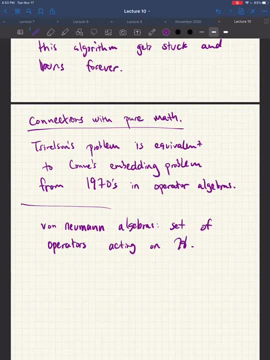 So it's a set of operators on H. you know, since it's an algebra, you can add and multiply them and it all lives in this algebra Right. So you can imagine it's like this giant, infinite bucket. The operators: 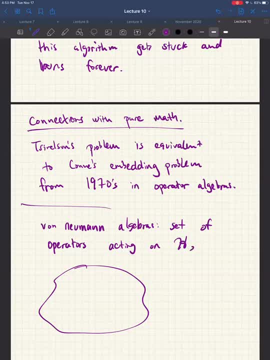 And it also satisfies some closure properties. Okay, So this is really abstract kind of thing. Multiplication also contains limit points, Right? So I guess this is sort of the defining feature of von Neumann algebra, Like if you take a sequence of these operators. 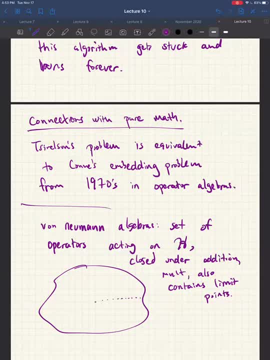 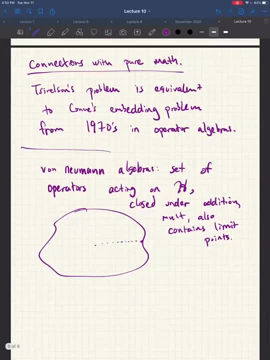 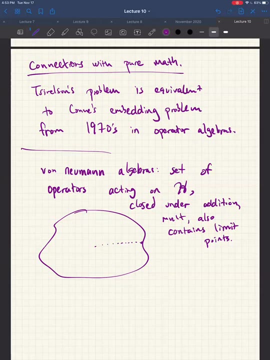 these the sequence, will you know, if it has a limit in some appropriate notion, then this set will also contain that limit, Right? So anyways, just that, that's how we can think of this von Neumann algebra, And in this subject people care a lot about classifying all the different types of von. 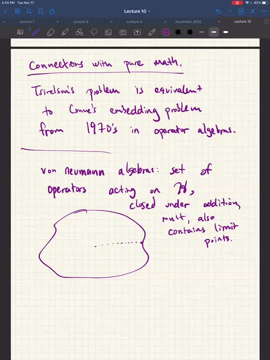 Neumann, algebras out there, Right And, and it you know it's really serious mathematical work. Right, mathematical work to try to figure out, like, what are the different types And this con embedding problem, the CEP. 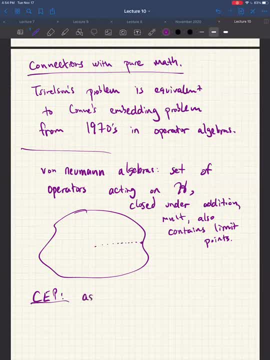 it asks whether there's a certain class of von Neumann algebra. is called type two one. Okay, so very scary looking nomenclature. So this is a certain class, whether they can all be. can all be embedded in a very specific von Neumann algebra? 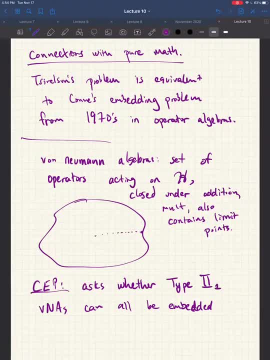 Something that's very nice that we have a pretty good handle on. Okay, so technically speaking, it's not just embedded in this thing, but technically an ultra power, whatever, that is, an ultra power of the hyperfinite algebra. Okay, so what's the significance of this? 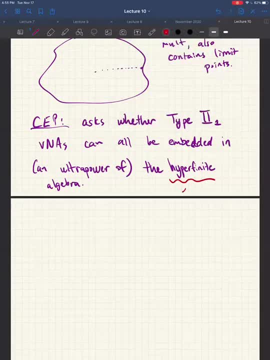 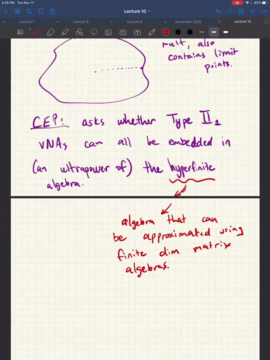 This hyperfinite thing. it's really nice because basically we can think of this as representing the algebra. that is where you can approximate it using finite dimensional stuff. Okay, and you can maybe start to see why this would be really nice, right. 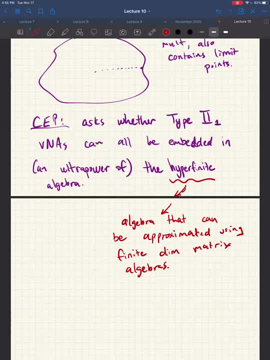 Like you have all these really abstract things in there, super crazy and infinite dimensional, but if it turns out they can all be viewed as instantiations of this hyperfinite thing. then it says: well, all the tools, all we need to understand that they're just. 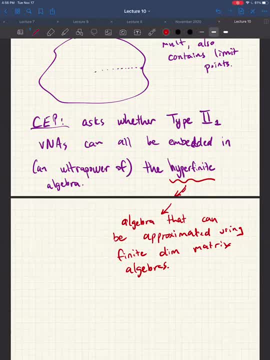 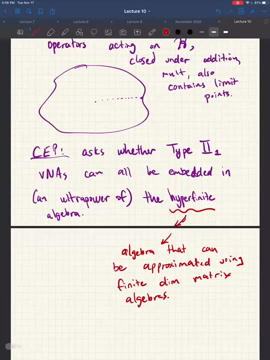 it's finite dimensional approximations, And I think we have a pretty good handle on finite dimensional matrices right. They're very concrete and we have a good feeling for them. So mathematically, this would have been a very nice outcome, And this was a question that was asked in the 70s. 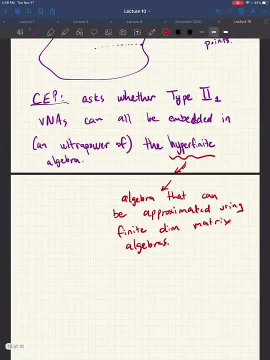 whether this was true, And so this started off in operator algebras, And over time people realized that it's actually something that goes beyond functional analysis. Like people discovered that there are equivalent formulations in group theory, in ergodic theory and in many other parts of mathematics. 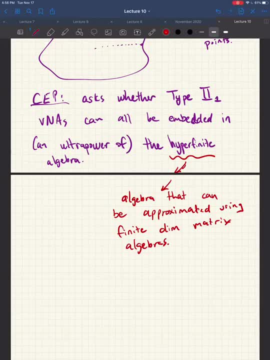 And it turns out that all of these questions are equivalent to each other, right In, maybe a surprising way. And all of these questions all have the flavor of: can you approximate some infinite dimensional thing using a finite dimensional object And one of these equivalent formulations. 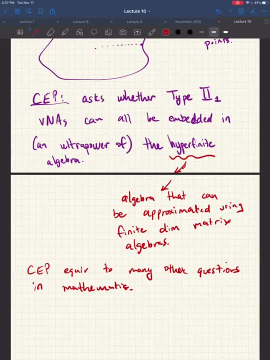 was the serial sense problem right In quantum information theory. it turned out that it's equivalent to CEP. So that's kind of a very curious connection And it's sort of like surprising and mind bending that this we started with something just about. 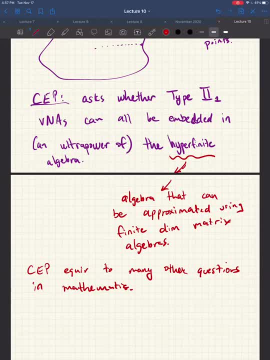 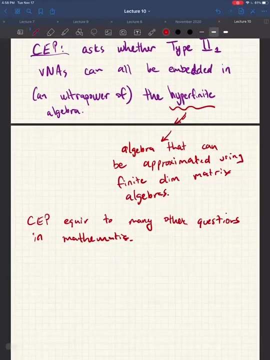 is there an algorithm to do something? And it's not related to this very abstract, deep question. in pure mathematics, It's more of an abstract question. So if you're looking at the, so if CEP is true, then omega star is equal to omega co. 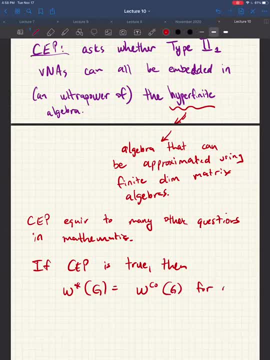 g for all, g right. In particular, this would, if CEP is true, then there is an algorithm And so, if you're looking at the equation, if you're looking at the equation, an algorithm for non-local games. Actually, does anyone actually know what the von Neumann? 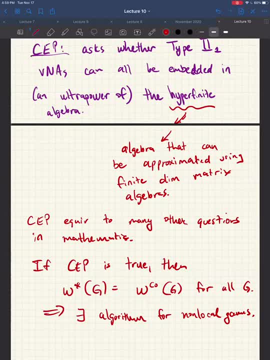 algebra is or has taken a class in this stuff? I notice that there are some math students at some point. All right, Randy, are you covering this sort of stuff? This is a prereq for the course that uses it. Sorry, I didn't get that. 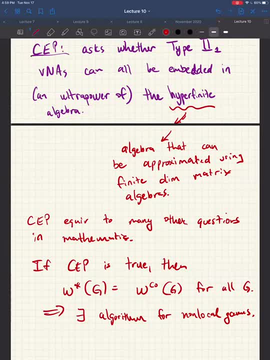 This is the prereq for the course. Oh, it's a prereq for the course. OK, Hopefully taking the next term, OK, so, yeah, maybe this is a good breakpoint. So let's come back in. let's say five minutes, like 5.05.. 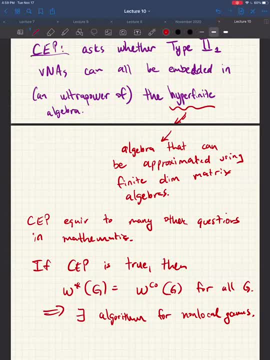 And we'll start to see. how do you disprove the existence of this algorithm? So I'm going to ask you a question And then I'm going to ask you a question in the meantime. So I'm going to ask you a question in the meanwhile. 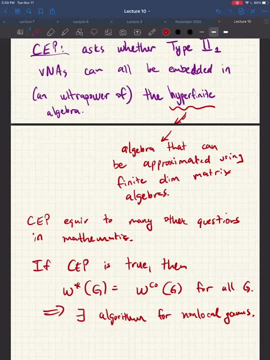 So I'm going to ask you a question in the meanwhile. Hey, Henry, can I ask a question in the meanwhile? Yeah, what's up? So I'm a little confused. So wasn't Serilson's problem already implied by Slavstra's result? 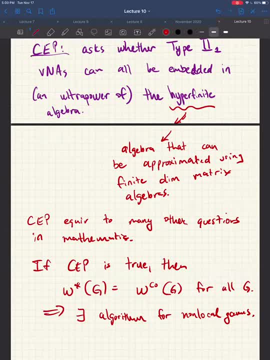 And so why did it take until the proof of MIP star equals r? e to disprove? But I know something's off, right? Yeah, good question. So actually there's multiple Serilson's problems And I think the Serilson problem that I'm mentioning 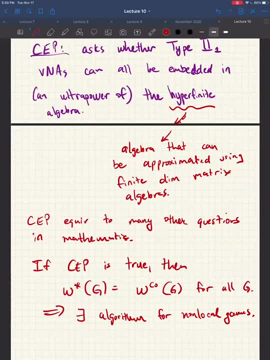 was the original one, But then over time, people came up with more fine-grained versions of them. And what Slavstra's result? what Slavstra did was he created a separation between two other correlation sets. So basically, he showed that there's a game. 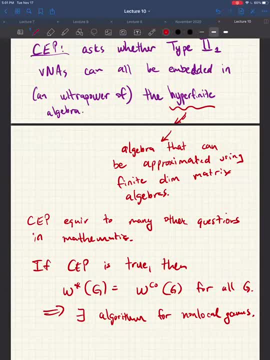 that you can come up with where, if you look at the sequence, the limit of all finite dimensional strategies, there is a particular limit, like the winning problem. So in the limit the winning probability is 1. But there is no finite dimensional strategy. 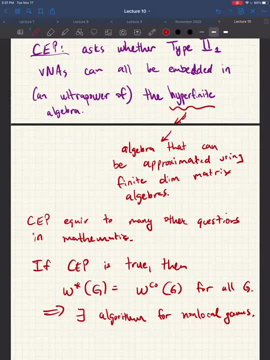 that actually achieves 1. Right, And this is not the one that CEP is equivalent to No. So CEP would say that here it doesn't insist that there is something achieving The limit. So basically, this is saying that it's. 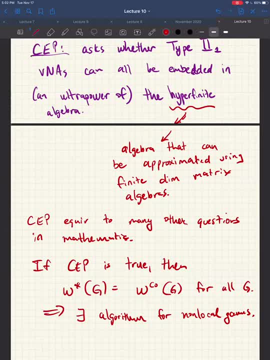 like the difference between a gapped result versus a non-gapped result. So if there is a difference between omega star and omega co, it would say that with commuting operator you can win with probability 1.. But even if you take the limit of finite dimensional, 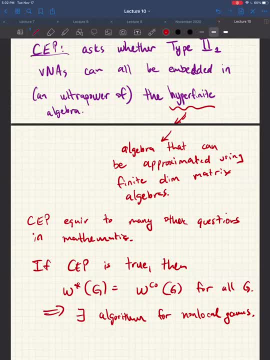 strategies, you'll get a lot more. So if you take the limit of finite dimensional strategies, you'll get a lot more. But if you take the limit of finite dimensional strategies, you'll get a lot more Because you're looking at a limit that's strictly less than 1.. 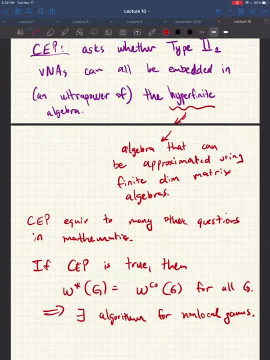 But you're looking at a limit that's strictly less than 1.. Hmm, That's a subtle difference. Yeah, Yeah, Right. So the other one is just, I guess, saying that for omega star you need the supremum rather than 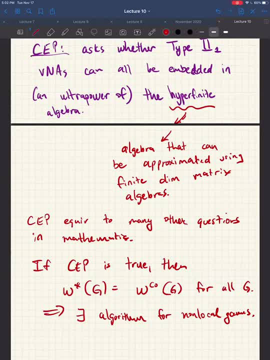 a maximum, But the problem we're talking about now is that you know, I was saying that even if you take a supremum, you still have this gap. Yeah, So I think that's a good point. So can I come back to a question I asked earlier? 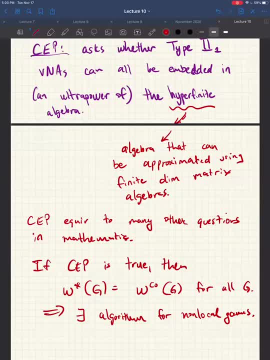 Which is OK. we haven't proven the result But if I'm understanding right, we have said that there is some game such that omega star is not equal to omega co And I'm not Like before you kind of hedged when I asked. 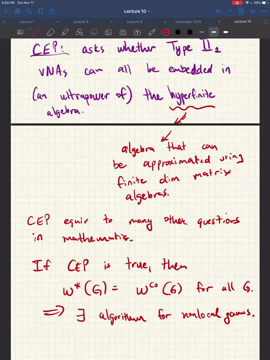 why do we not take that as a definitive answer to whether the world needs to be modeled as infinite dimensional Mm-hmm? So can we take that as a definitive answer that, yes, we actually do need infinite dimensions? I'm still not sure. 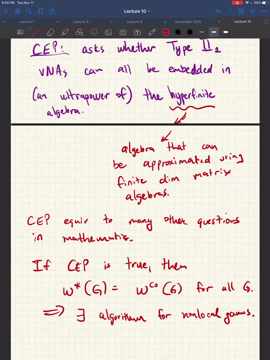 I mean, it's just related to some of the things that we've been talking about, which is that, you know, maybe it's just not physically possible to play this game and achieve this omega co value, In which case, you know, you could argue that maybe still. 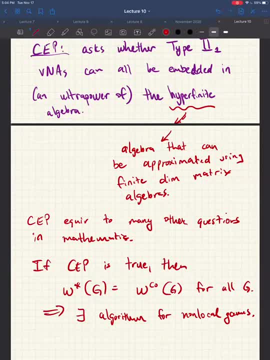 you don't need, OK. But the only reason that would be the case, if you know, once we say make QFT rigorous, would be because the game doesn't satisfy. you know some property of that. But supposing that it does, which I think- 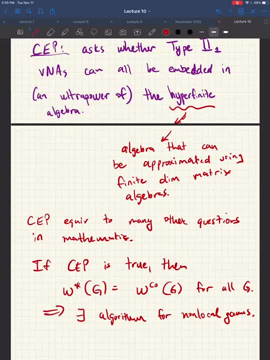 is kind of what we should believe at the moment, then the answer to that question is yes, You know, to the best of our knowledge, we need to model the world as infinite dimensional. Mm-hmm, I guess it would tilt the needle more in the direction. 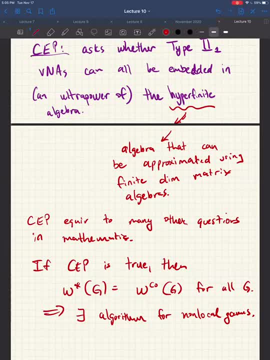 At least, OK, my opinion. I think it would tilt the needle more in the direction of what you're saying. But you know, you can still. You can still raise possible valid objections to whether you know if there's a technological obstruction. 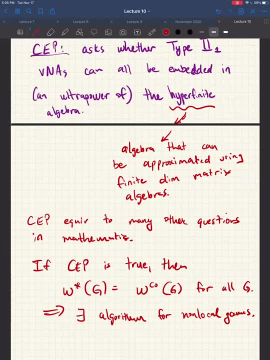 like you know, let's say I don't know because of, like you know, the configuration of you know, like the only way to conduct this experiment is if you collected so much mass in like a very compact area that it would like create a black hole or something. 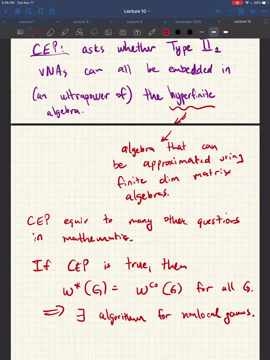 Uh, You know, maybe you'd say: OK, Actually, maybe it's not feasible on physical grounds. Fair enough, Thanks, OK, so let's continue. So let's jump in to see, like, how is this non-computability? 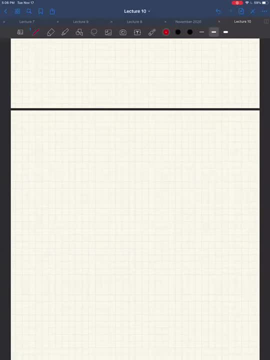 result proof. So this is the content of this result: MIP star equals RE And the main statement of the results is that there exists a computable reduction or transformation from From From From From Turing machines, From From. 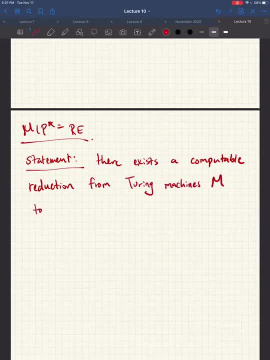 Turing machines, From Turing machines, From M to a non-local game, G sub-M- such that if M halts, then the omega star value of this game is 1.. If M does not halt, Then the omega star value would be 1.. 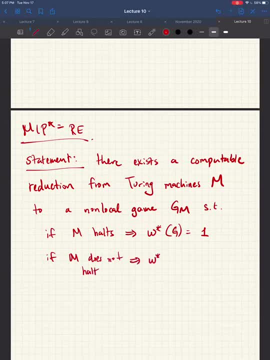 So you just have to keep that in mind. If a non-local game G sub-M, Such that If M halts and the omega star value of this game is at most a half, So a Turing machine, you can just think of it as a computer program. 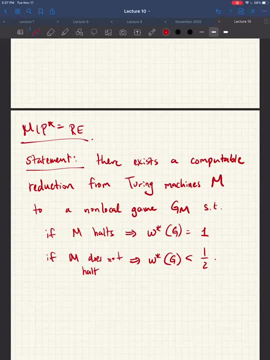 it's an algorithm. I like to think of it as something you write in Python, so something very concrete. right? Someone hands you a Python program, then the statement of this result says: I can convert this Python program into some non-local game. 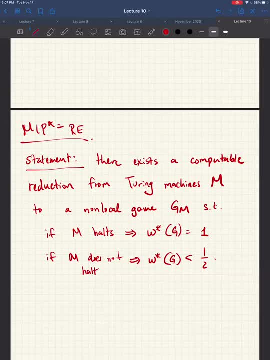 where. imagine that you just ran the Python program and if at some point the program terminates, then the omega star value of this game is one. but if your Python program gets stuck in an infinite loop or it just never stops, then the value of this game is at most a half. 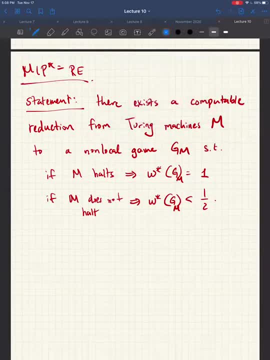 And so the first thing we should argue is: this implies there's no algorithm. there's no algorithm to approximate omega star to something less than a half, Because if you could approximate this value to within a half, you could determine whether an arbitrary computer program 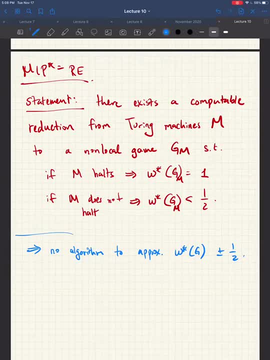 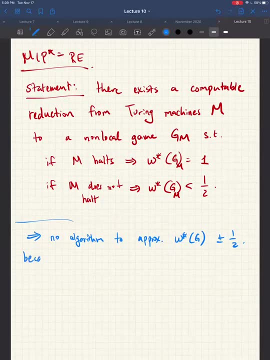 halts or does not halt, And this is something we know is not possible. Okay, All right, and I'll say a little more about this in just a second. we've kind of been alluding to this the whole time, but let's just unravel the consequences. 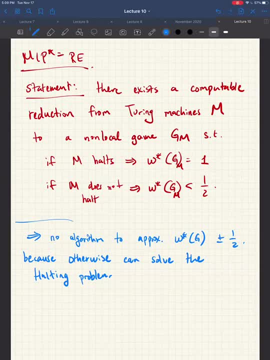 There is no algorithm to to approximate this game value, in particular the algorithm, uh, that i described, that does a search from below, search from above. it cannot work, uh, which means that, um, you know, there's a negative answer to serosin's problem. um, right, so there's some game like. this statement doesn't. 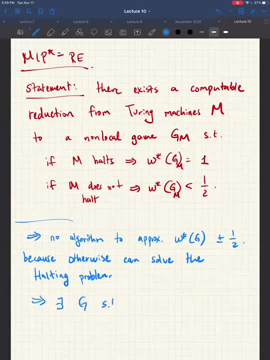 tell you what game it is, but there has to be some game g, uh, such that um omega star g is different from omega co, so so that's pretty interesting. um and in particular, like for this pure mathematics application, um, there exists these type: 2: 1 von neumann algebras. 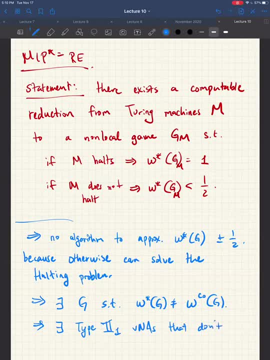 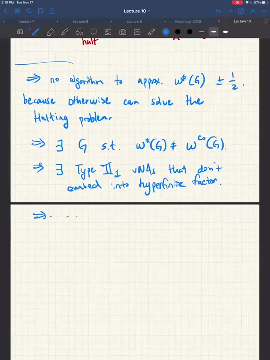 that don't embed into this hyperfinite factor, right and you know. and then, like you can knock the dominoes to all these other connections to these area, other areas of mathematics, um, so called a c-sharp algebra, say something about uh this, uh right, uh, so, fortunately, 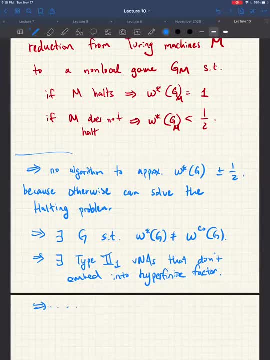 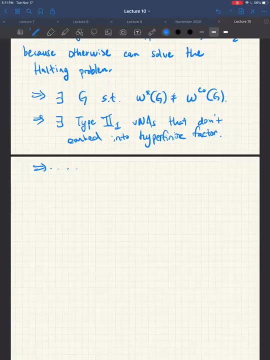 the all of this does not depend on your choice of programming language. um, it's all you know, turing equivalent. um. okay, so to uh, just to sort of like prime ourselves for like how we should think about this. i'm going to quickly go over the proof of why the halting problem is not solvable. um, probably many of you 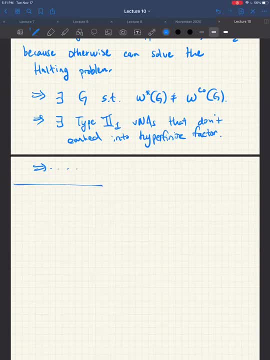 have seen this already, but i think, um, it'll be helpful to just review. um. so the halting problem, right is, it's just to determine whether a given computer program halts or not. so you're given the description of a turing machine. uh, m determine whether it halts. 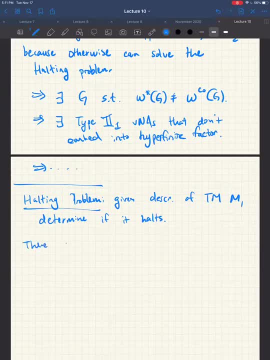 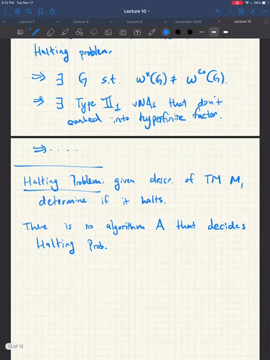 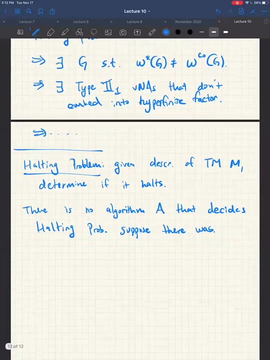 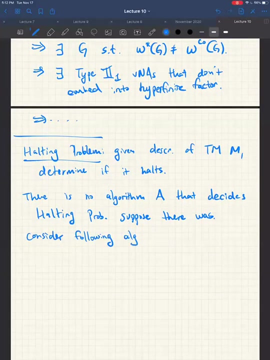 okay. so, um, there is no algorithm a, uh to, to determine this right, and um, we'll prove this by way of contradiction. you know, suppose there was. then we're going to create a self-defeating algorithm. you know that creates a contradiction between the two. so i'm going to call this algorithm b. so what does b do? 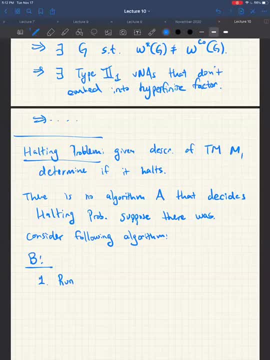 it's going to run this supposed uh halting solver on input b. okay, so, in particular, it's going to run it on its own source code. okay, and first, um you know you, if you haven't seen this before, this might seem kind of suspicious- like how is it possible to to run another program on yourself, right? um, it turns out that it is uh. 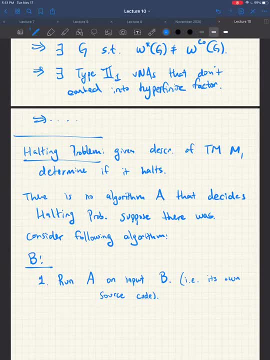 like you, you can actually do this and um, i think that's kind of where it's going to get. a little like you can actually do this and you know, if you're curious like how this is possible, you should. you can google something called the quine, right. so these are examples of computer programs. 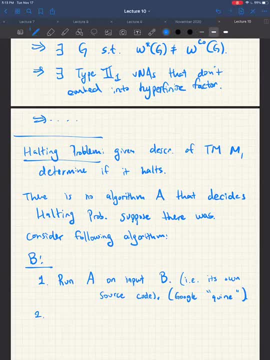 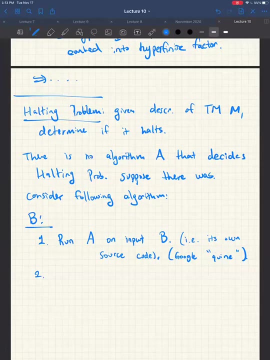 that print out their own source code. and if you've never tried something like this before, it's actually kind of tricky. so it's a fun logic puzzle but but it is possible to create these things. so in particular this step one is well defined, like it makes perfect sense, like in any 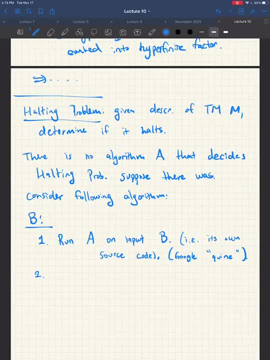 programming language you can do this. so you're going to run this halting solver a on input b and supposedly it's going to tell whether b halts or not. but we're we're just going to run this halting solver a on input b and supposedly it's going to tell whether b halts or. 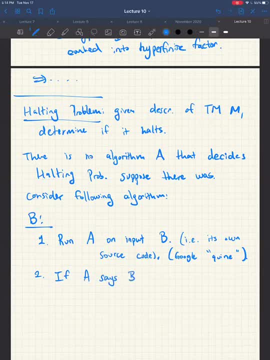 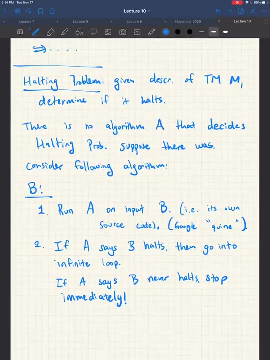 not, but we're, we're just going to do the opposite, you, okay? so this is our uh computer program b, and you know, uh, let's think about whether b halts or not. so so you know you say, well, suppose, like you know, for any algorithm it is just, you know, a god-given. 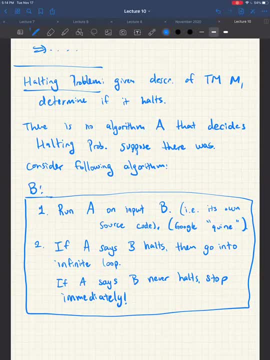 truth, whether it eventually halts or not. right, it's like a well-defined uh truth. so for b, let's say, uh, it's supposed to halt, but sort of by construction, it's supposed to halt, but it's supposed to. it will say, well, i'm told i'm supposed to halt, so i'm just going to do the opposite, i'll just get. 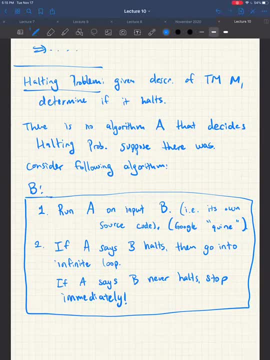 stuck in an infinite loop, whereas if a says b never halts, then i'll just stop immediately. so i actually do in fact halt and, and so you see there's a contradiction. uh, both ways. could it be? uh circular that b is defined on a like? shouldn't that not be uh allowed in your proof? 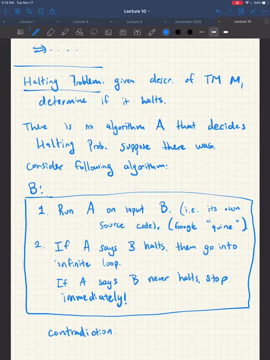 well, um, yeah, i guess. well, b depending on a is fine, because b and a are separate algorithms. but, like i mentioned, you know you could be suspicious of the fact that b is calling a on itself, but this is a legal thing, you know. you can't program- uh, you can write a computer program that that does. 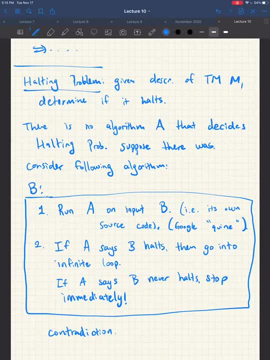 this because, i mean, computer programs are just like strings of characters, right? so it's basically you're saying you give it the string of characters that make up the program as input and so, like any, any program isn't going to be a finite string of characters. 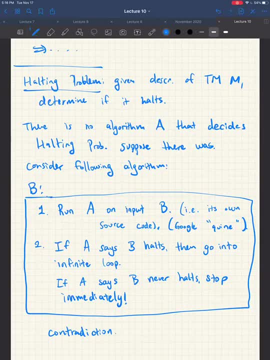 So you can just give it that string of characters as its input, Right, I mean, but it's not 100% obvious, because if you were to write this naively, you would say, well, input my own string of characters in this. 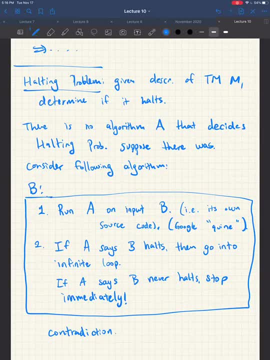 But you can't continue expanding out. You have to do something more clever to make that work out. But yeah, basically it comes from what Hugh just said. OK, so now this is like kind of a cute logic proof, But you notice that there's this element of self-reference. 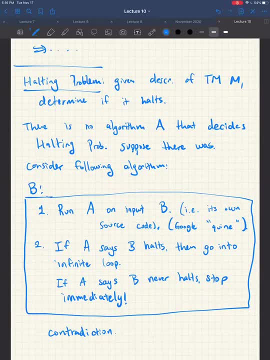 Like you have a program that's talking about itself And this is how you prove that the halting problem has no algorithmic solution, Right? So outside of this class of algorithm B, could you say that halting problem is solvable? So certainly there's lots of algorithms. 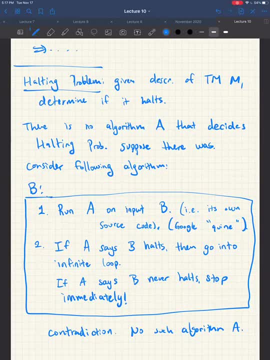 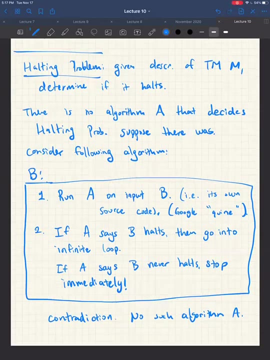 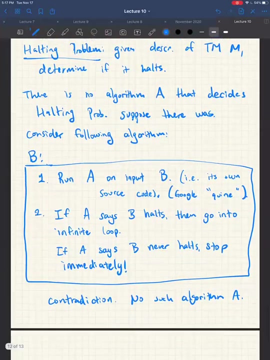 for which you can look at and analyze and try to deduce whether it halts or not. But what this argument is saying is that in general, you cannot hope to solve the halting problem for all algorithms, Right? Would this mean that? does this not rule out? 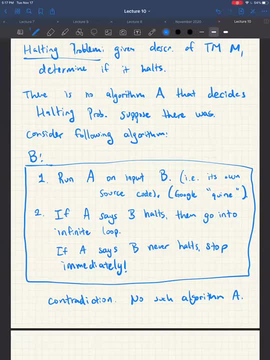 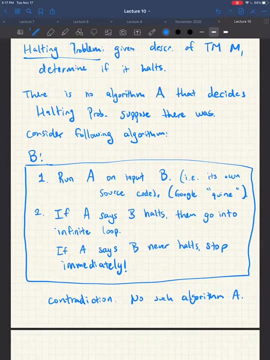 a algorithm that, let's say, solves the halting problem but also could also never halt. So in what sense do you mean solve? So like the Yeah, Yeah, Yeah, Yeah, Like if A were a run on itself, it will never halt. 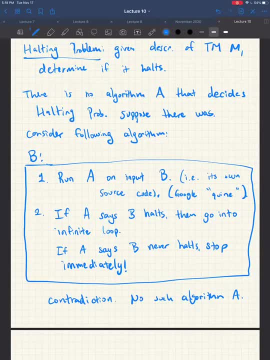 As in like it will never. oh, if A runs on itself, then it will never say whether A the input halts or not. Well, we don't know. I mean this algorithm A doesn't exist. We just proved it doesn't. 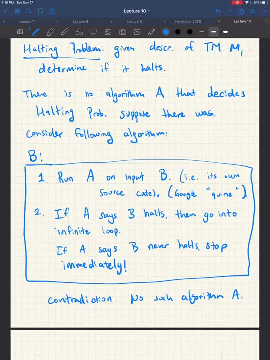 But I guess part of the proof says: well, assume that it did exist and, in particular, assume that A halts on all inputs. So presumably if you ran A on itself it would say, yeah, I halt. OK, then 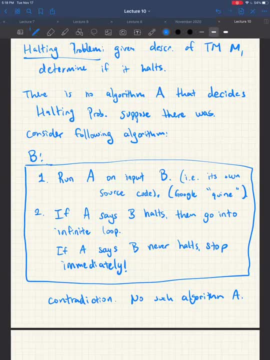 But you do point out something which is like, in some sense, if you wanted a semi-algorithm to solve the halting problem, you could. and that algorithm is very simple: Just run the program to see if it halts. If it doesn't halt, you just keep on running forever. 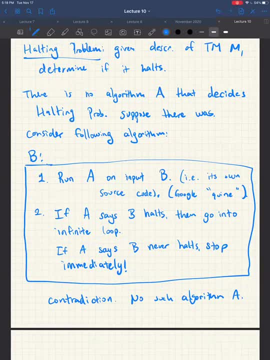 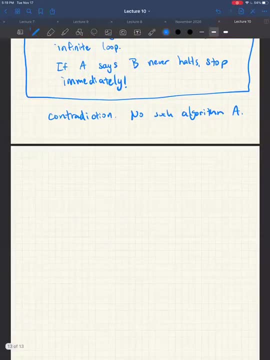 And in that sense you've kind of like semi-solved it, OK. So with that primed in our heads, let's see how do we take arbitrary programs and embed them into nonlocal games, And this comes through a tool called Compression of Nonlocal. 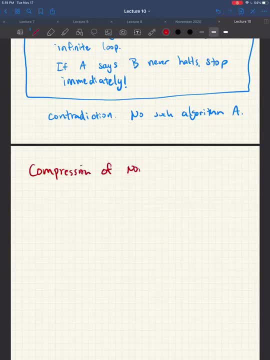 local games. We're going to use this idea of, you know, taking non local games and kind of like, just compressing them in a way that we can encode computations into them. But before that I'm going to have to do a little more setup, So to sort of make this work out. 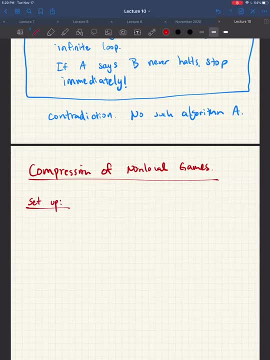 like we need some way of talking about games in terms of algorithms, right, Like we need some kind of like unified language. So this is how we're going to do it. You know, let's say that you know, cursive G or curly G is an infinite family of non local games. 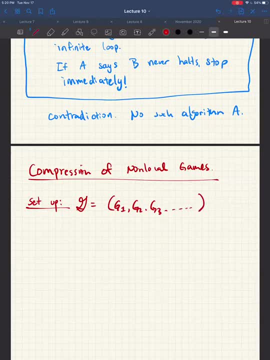 So it's not just one game but an infinite number. So each GN is going to be some non local game that has its own. you know, question and answer, alphabets has a question distribution, some decision procedure, right. So for every end there is such a non local game. And now 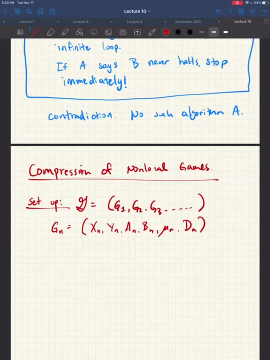 how they're all going to be related via a single Turing machine. So you know this thing. I'm going to call it a uniform game sequence. So uniform because there exists a Turing machine V, just a single Turing machine. that implicitly describes all. 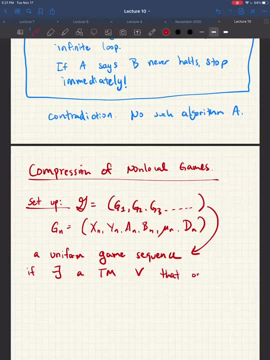 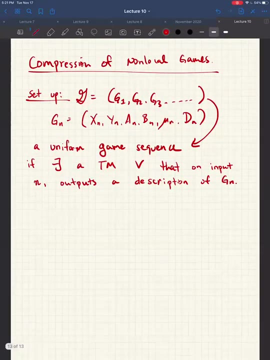 of them at the same time. Okay, So this V you plug in and it says, okay, here's what how the Nth game works. And what does this description look like? It's going to tell you the sizes of these question and answer alphabets. 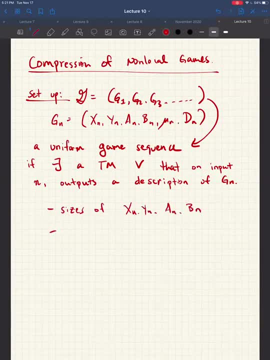 Okay, Okay, It's also going to give you basically a recipe for how do you sample from this question distribution. So this recipe will be in the form of another computer program And it'll give you this Other computer program, DN, that computes this decision procedure. 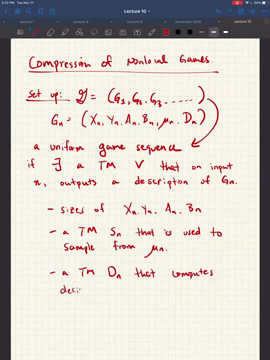 So you know, think of it this way. like you say, I'm interested in game number 100. So I'm going to go up to this Turing machine V, I'll plug in 100 and V is going to spit out a bunch of questions. So I'm going to go up to this Turing machine V, I'll plug in 100 and V is going to spit out a bunch of questions. So I'm going to go up to this Turing machine V, I'll plug in 100 and V is going to spit out a bunch of questions. 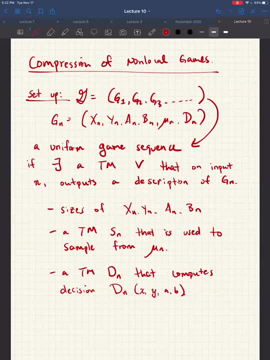 And this data will be everything I need to know in order to execute this game. So you know, imagine that I'm the verifier and I'm playing with Alice and Bob. You know, given this description, I can use this S sub N to choose my questions at random. 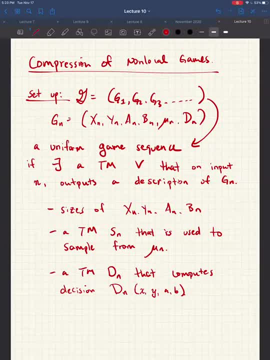 So I'll run this Turing machine. it'll help me choose these questions X and Y. I send the questions X and Y to Alice and Bob. They give me answers A and B And then to figure out whether they win or lose, I'll just plug all the questions that they've given me. 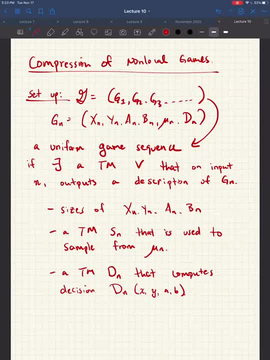 I'll just plug all the questions and answers into this D sub N Turing machine and it'll tell me whether they won or not. Okay, so it should be clear that this V tells you everything you need to know about this sequence of games. Now, to make this like kind of meaningful: 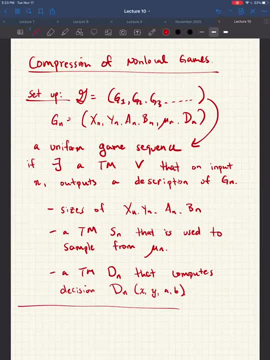 we also have to insist that everything's computable efficiently. So everything has to be computable in polynomial time Right, and this includes, like running this Turing machine V right To get the descriptions. it has to be. I have to get the description. 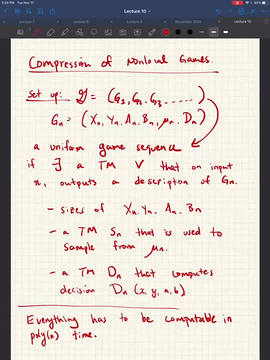 in some reasonable amount of time. So poly N time Once I get the descriptions. when I execute the game- like sampling the questions and deciding whether they win or lose- all of that has to take polynomial time. Why? why is it not enough for this to be computable? 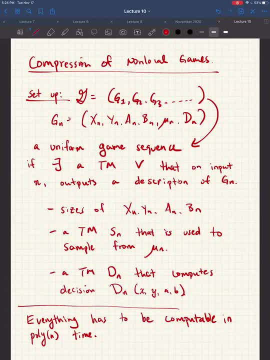 Good question. I mean a priori, you don't have to insist on this. but in this compression argument we're going to actually have to keep track of how much time things take And it gets. it's not so important whether it's polynomial or something, but just. 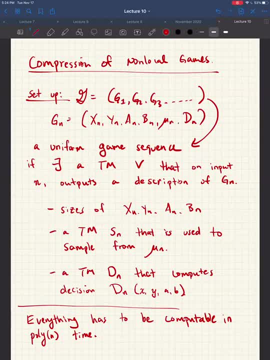 we just have to have a handle on what the complexity is. So SN, I guess, would have to be a Turing machine with access to random bits. right, You can think of it that way. I mean, I haven't exactly said, you know. 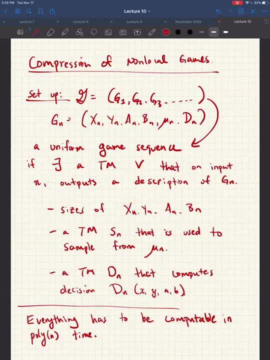 how does it tell you how to sample? but you can imagine that it's some useful way of sampling from it. So, yeah, you feed in random bits and it'll generate a sample. yeah, Okay. So actually, like you know, 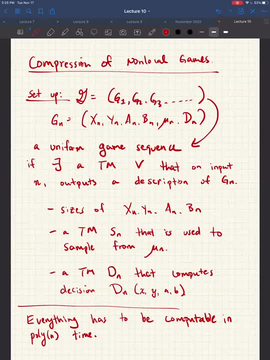 we won't talk about this today, but in the proof there. there you know, SN will tell you more details about the distribution that they'll be helpful. It's not important for now. Okay, so that's one setup We have a way of talking about. 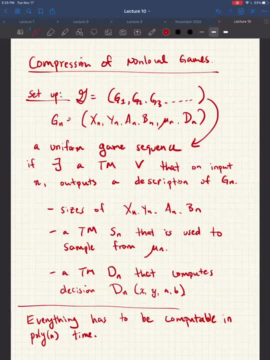 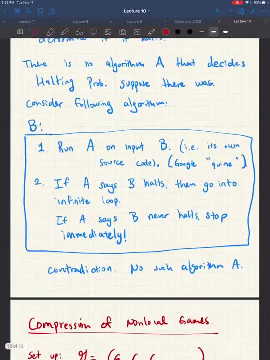 I'm sorry, was there a question? Yeah, I was wondering, just like going back to the like halving problem for a second, Uh-huh, Like kind of confusing, Like if you ran an algorithm- or is it even like a legal algorithm, one that like basically says: 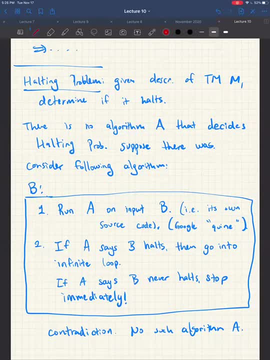 like if, and then some statement that like is like a contradiction, like is neither true or false, Like if, this statement then like go in an infinite loop. Otherwise, like halt, like something that wouldn't even either halt or be, or go into an infinite loop, you know. 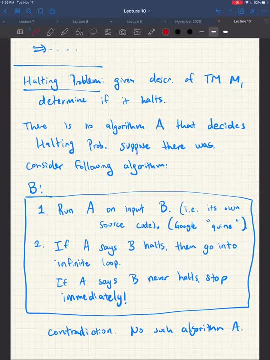 Like it wouldn't be either, but like, okay, either of those options, because it's like saying something that isn't neither true or false, Right? so I guess here we're sort of doing, we're playing this game which is like proof by contradiction. 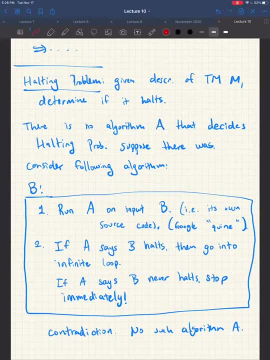 So we're assuming that this algorithm tells you a well-defined answer. like it says: outputs one if it halts, output zero if it doesn't halt, And we're guaranteed that, by assumption, this algorithm A will always output zero or one, regardless of what you ask the algorithm. 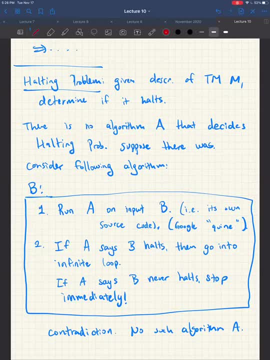 So this: if statement is well-defined, right, Like it either output one or output zero, And depending. if it's one, then I'll do something, If it's zero, I'll do something else. What about like an algorithm that outputs zero, one or two? 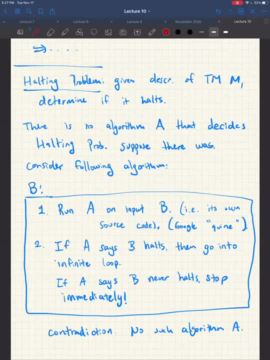 if it's impossible to output zero or one, Oh sure, So that's well, you could say- I think it won't be so important for this argument- Like you can say, if it outputs one, then go into infinite loop. 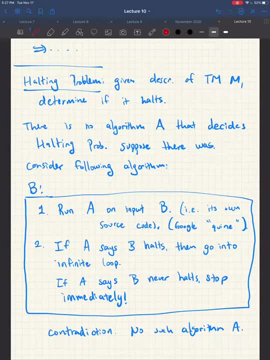 If it doesn't output one, if it outputs anything else- zero or two or three or whatever- then halt. And you still run into a contradiction. Okay, thanks, Yeah, yeah, I mean this halting problem. proof is one of those things. like it's simple. 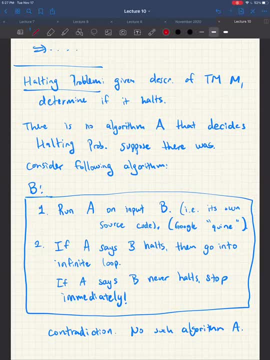 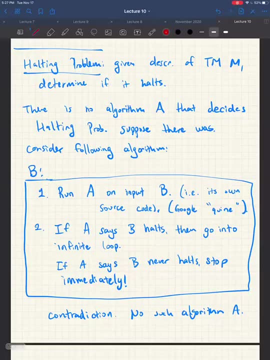 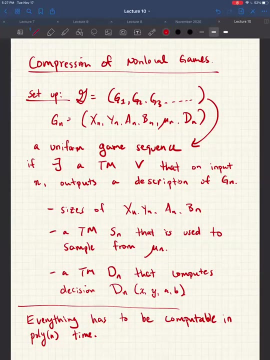 but you could just kind of have to dwell on it for a while. Yeah, just wait till you see how we use the compression theorem, which we'll get to in a second. Is everyone good with like this V and describing this infinite sequence of games? 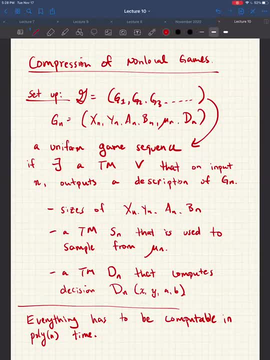 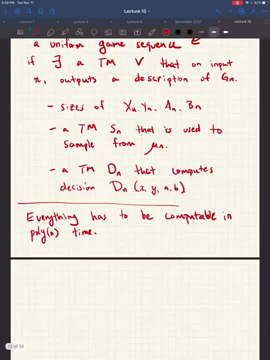 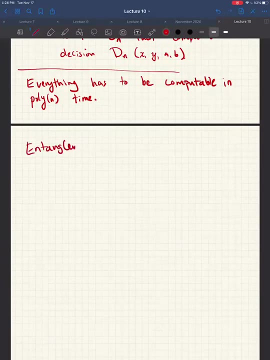 Hopefully it should be kind of intuitive. It's just some way of describing an infinite family of games. Okay, I just need one more piece of notation, And this is gonna be something called the entanglement lower bound. And so this is: you fix a nonlocal game G. 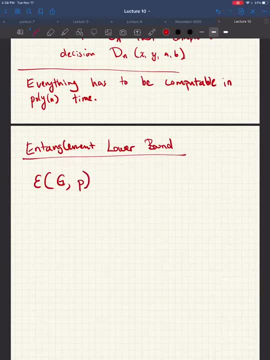 not a family of games, but just a single nonlocal game, G, and you fix a probability P and this E of GP is going to be a number, it's the minimum dimension D, such that using a D dimensional strategy, you can win in this game with probability at least P. 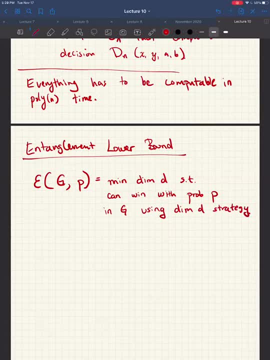 All right, And if there is no such finite dimension D, then we just define this number to be infinity. Okay, so it's just saying, it's just measuring, like, what's the minimum size dimension you need to win with any particular probability? 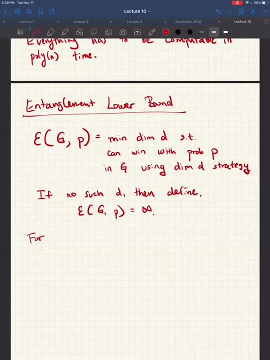 So you know, for example, let's take our favorite CHSH game. You know what are the entanglement lower bounds. So for three quarters, what is this? quantity Zero, Zero, yep, Cause you don't need any entanglement at all. 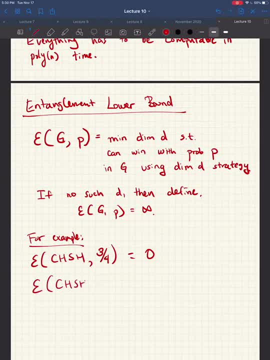 You can just use a classical strategy. What about this? What about this? What about this? Cos squared Pi over H. This is One, One or two. I mean, it's something. technically it's two dimensional, but- Okay, oh yeah. 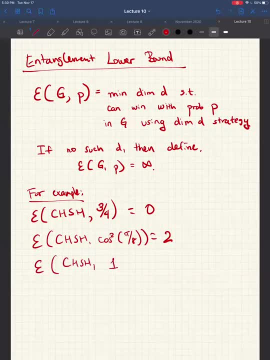 Yeah, And for one, this is going to be Infinity, Infinity, yeah, Cause I mean, this is Cirylson's bound that we saw a few lectures ago. right, there's no probability, one strategy, Okay, so that should make sense. 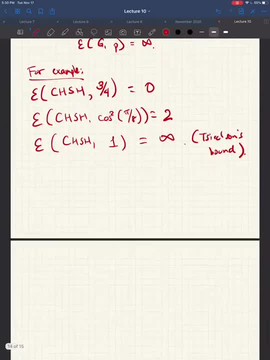 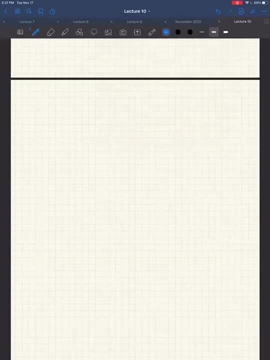 All right, so now for the heavy hammer. this is gonna be really like the main technical thing. Let's see the statement of the compression theorem. Okay, so this is going to give us a procedure for compressing an infinite sequence of games into another infinite sequence. 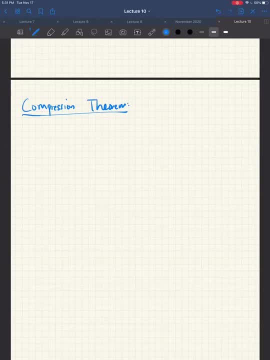 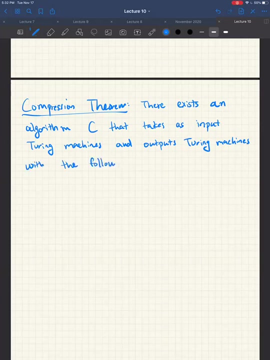 that is compressed in some sense. So here's the statement: There exists an algorithm C C for compress that takes as input Turing machines or algorithms, and outputs Turing machines. okay, With the following property, All right. so the way I like to think about it. 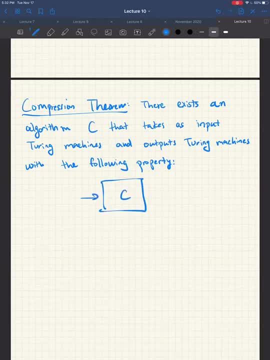 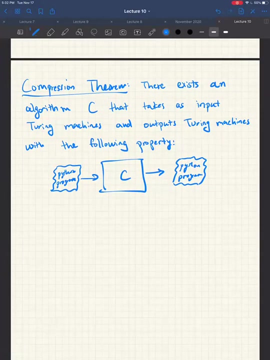 it's really this box and incomes. you know a Python program And it'll do some crunching and it outputs another Python program, All right. So what are these Python programs? So let's say that you know. let's call them V and V prime. 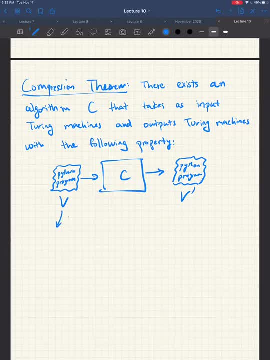 V is going to specify. you know, V computes some infinite sequence of games in the way that we just described, right? So suppose that you gave this V and it describes the sequence of games. then it'll output another V prime that computes another. 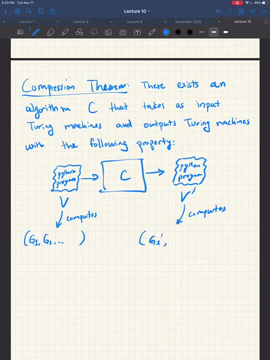 sequence of games. I'll call it G1 prime, G2 prime, et cetera. And now I have to say: how are these games related to each other? For all N if Omega star of the N plus first game of the original sequence. 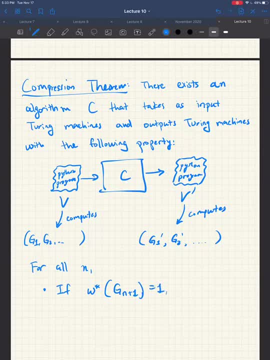 is equal to one, then the Nth game of this compressed sequence is also equal to one right. So in some sense this compression procedure preserves perfect winning probability. And the second thing is we have a relation between the entanglement needed. 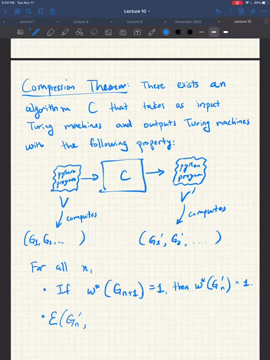 and the probability needed to play this compressed game. with probability a half It's at least the greater of either the entanglement requirements for the N plus first game of the input sequence or N. So I think I can see why you want the first condition. 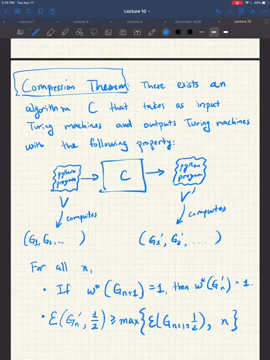 because you will construct a series of games that if the Turing machine holds, then from this point on it will stop on. the probability to win will be exactly one. and then you just compress again and again, and again and again. But why do you need the second condition? I'm not seeing. Well, we'll see in a 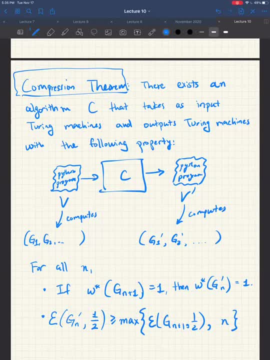 sec, but I think, yeah, you're on the right track. Yeah, so I think the the salient features are that, first, it's a transformation from a sequence of games into another sequence of games, such that the second sequence is related to the first in this kind of shifted way Like we have this. 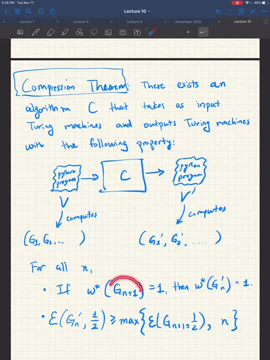 the nth game of this second sequence is related to the n plus first game of the original sequence and we have this somehow. the entangle- whatever entanglement you need- for this second sequence- is related to whatever you needed for the first sequence. 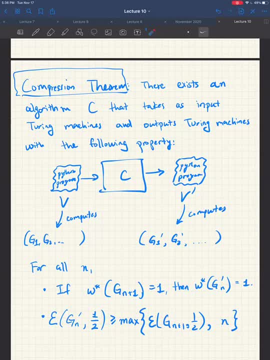 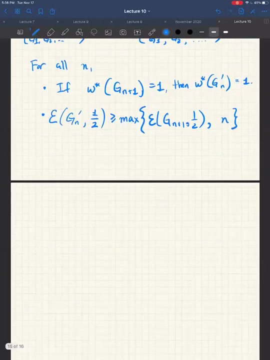 Yeah, so before I move on to show how this is used, any questions about the statement? Okay, so let's, we're going to use this to right. I told you that the statement was: I can take any Turing machine and map it into a non-local game, g, sub m with the, you know that can tell apart whether it. 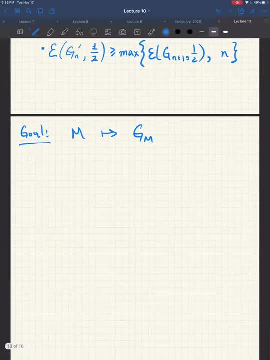 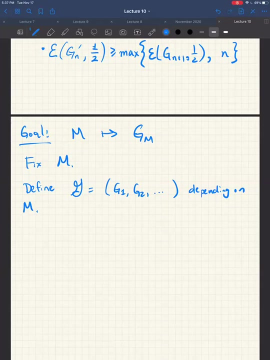 m halts or not. So let's fix this m right. We're going to use in order to define a uniform game sequence that depends on m, And the way I'm going to describe it is to use, you know, some bit of pseudocode. 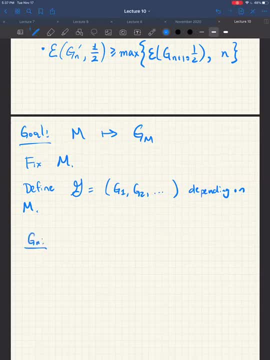 is how the nth game is going to work. It's just some informal description of how the game works. So imagine that you're the verifier in this nth game. So as the verifier, before you even talk to Alice and Bob, you're just going to take this program m and you're just going to run it for. 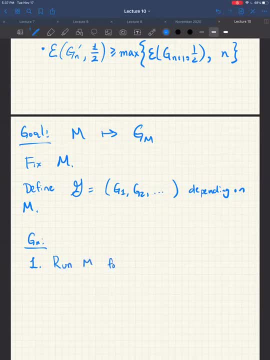 m time steps. When you say verifier for the game, you mean like the decision procedure d. Yeah, I mean like the combination of the sampling and the decision procedure d. Okay, Yeah, you know, just yeah, okay. So you know you're going to run m for n time steps. 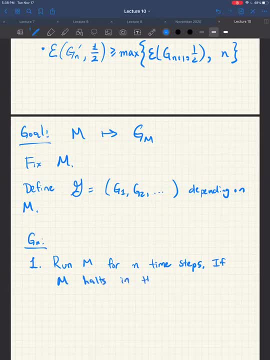 if m halts in this time, you say, great, except. So here you know. even before you've even talked to Alice and Bob, you say: well, you automatically win, right, I don't even need to send you any. 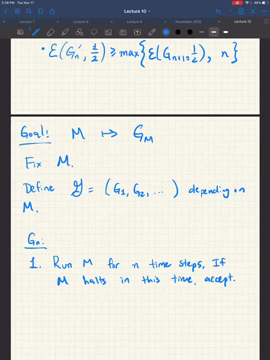 questions or answers. You know, go home and enjoy. But suppose that they- you know this Turing machine doesn't finish in this time, then the verifier is going to do something more elaborate. It's going to run this compression procedure c on v. Now what's v? v is supposed to be the Turing machine that outputs. 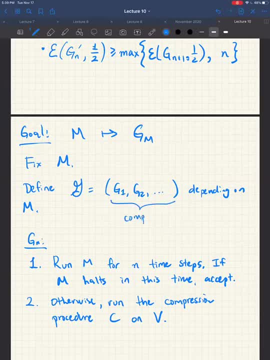 that computes this sequence and you might start getting a little weirded out by that. but we'll deal with this in a bit, in a sec. You know V is a Python program. We plug it into this compression procedure. C- Obtain V prime. 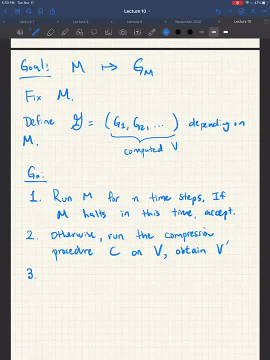 Okay, So now we're able to play with this output sequence: Run V prime on N to get a description of G prime N- some other non-local game right, And then, since we know everything we need to know about this game, we'll just play G prime N with Alice and Bob. 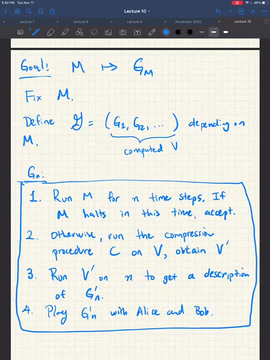 Okay, so you know. so I've just written some pseudocode down. The first thing I want to try to convince you is that this does describe a non-local game, right, Because you know you can imagine that the decision procedure. 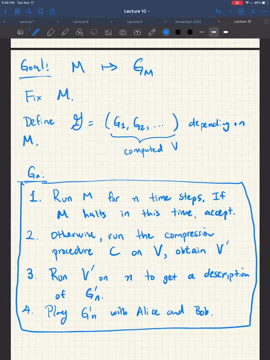 of this G N will sort of carry out all of these computations. Right, it'll run this M, it'll run the compression procedure, And when it gets this description of G prime N, it'll just do that. There's this funky thing of that where, in describing it, 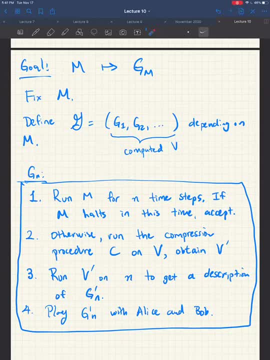 in describing G, prime N or, sorry, in describing this G N where we're saying: run this compression procedure on V. What's V? V is the thing that's defining G N, right, So there's like some circularity going on. 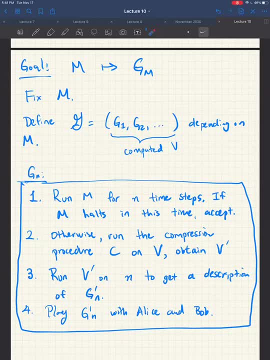 but it's the same kind of circularity that went on in the halting problem. proof: I claim that this is okay, Like we don't have to worry about it. it's well defined. Like this: all can be set up in like a self-consuming way. 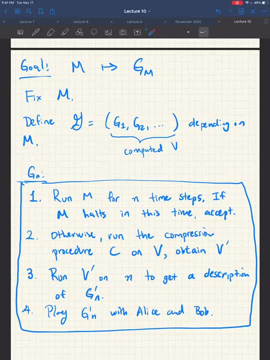 like a self consistent way, What else? Oh yeah, And so you know basically the fact that I've kind of written out this description, the pseudocode for you, like it's basically like the pseudocode of V, like when you run V, you'll output this description that I've just written. 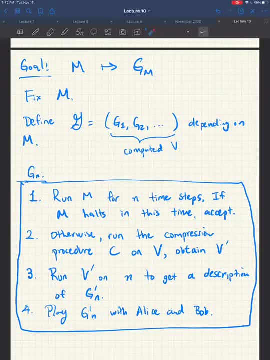 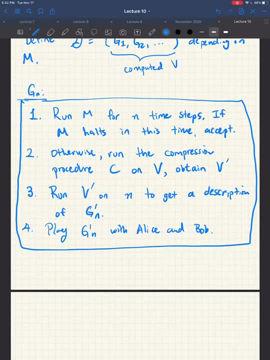 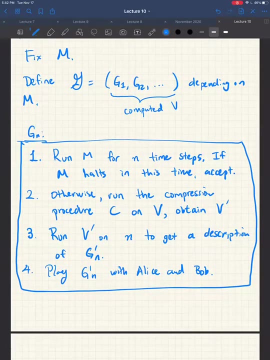 down for you, Right? So you can imagine that this is all possible. The other thing that I want to convince you of is that this sequence of games is all computable in polynomial time, Right? So let's just do an accounting of what's the time. complexity of each game: GN. 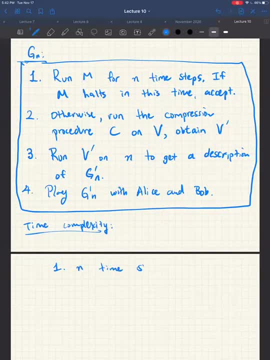 Right. So step one, you know, takes n time steps. right, by definition. Right, We're just running this program m for n time steps. Step two takes O of one time, a constant amount of time. Right, We're just running this. 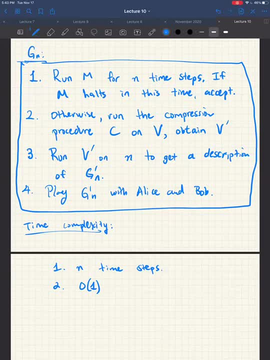 compression procedure on V. V is some fixed object that doesn't depend on n at all, And so when we compress it it just takes some amount of time. But the important thing is it just doesn't depend on n V prime. you know sort of we're guaranteed since it's specific. 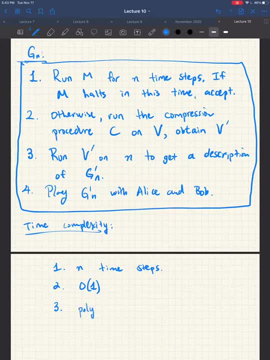 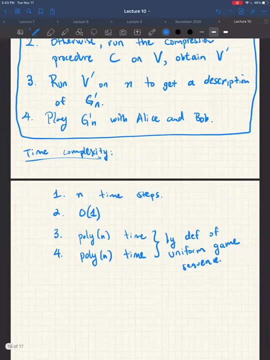 it just identifies like a game sequence. It runs in polynomial time. Also, this compressed game, G prime n, it's also going to be polynomial time. This is, by definition of uniform game sequence. Okay, so you know, we add all of this up and we get a polynomial time computable game. 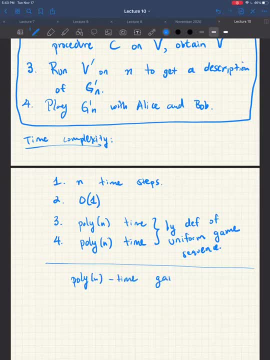 Especially if we can't trying to make the four nel whipped in, even if we have to do it in a more general way. Mm-hmm, I mean, some of these things make sense to us. I mean, this is my first time using it and I'm quite surprised by the. weren't you able to do this? 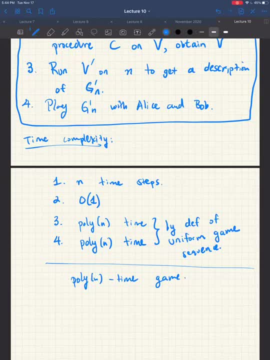 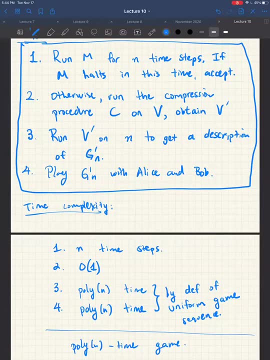 Why can you necessarily run C on V? Because doesn't like being able to run C on V depend on V being one of these. like be an algorithm that computes these kinds of game sequences, but only computes these game sequences if you can actually run C on V. 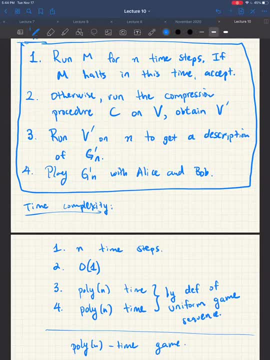 Yeah, so you can sort of set it up where, like you know, you first define it so that, no matter what, all of these games, gn will be well-defined, so v will actually exist. And so once you've set that up without relying on any other assumptions, and then once you've 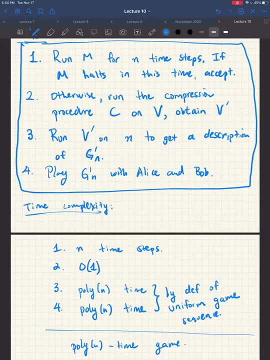 set that up, then you know that once you run c on v it will output another proper game sequence. So you find like a v prime prime and then you define v based off of this v prime prime, for example Something like that: 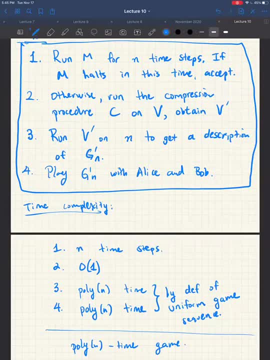 Yeah, you can do it that way. I guess you know at a high level this property of being like something that outputs a uniform game sequence. this is just a syntactic property, You know. it's not something that you have to like. run the Turing machine in order. 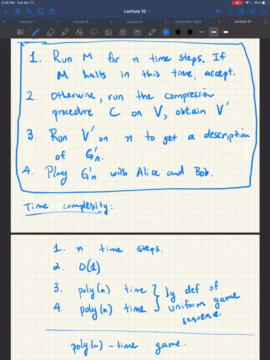 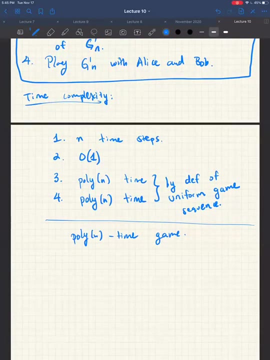 to find out whether it outputs a game. It's just no matter what the way the Turing machine is set up, it always outputs a description of some game. Sure, yeah, Yeah. So, depending on the definition of that g game arm. 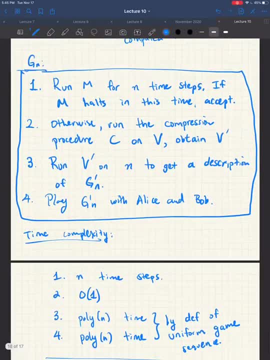 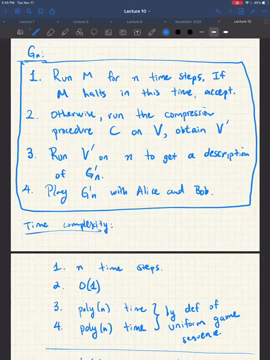 Is it possible that when you carry out your compression, that you can lose a lot of information on your v and that your v prime is not going to approximate v very well, especially if it has a lot of values that are well. it's called. the expected tensor is about the max. 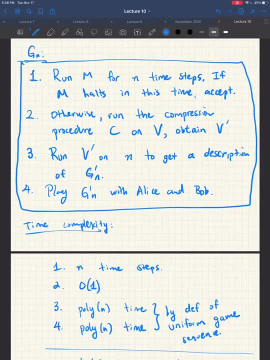 value there- max of expectation- and then that therefore c could, is a class of v, definitely, So the definition is that c could not be an optimal transformation to carry out on. I hope that makes sense. I didn't quite follow, but I guess the only thing that we'll use about this compression- 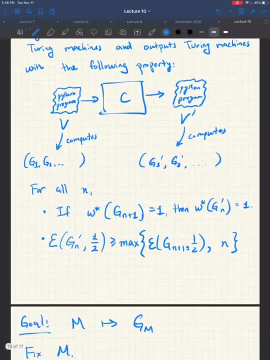 theorem are these two items that I've written down. So if the item of where you have the max there, the item on the left, is very large compared to the, say n value, Mm-hmm, Yeah, So the item on the left hand in the max is going to be much greater than n. 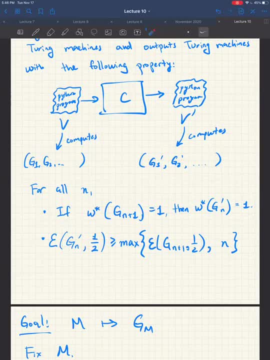 Could you wind up- and you have a lot of those values- could that then wind up with loss of information? So I don't know what you mean by loss of information, but all we know is just this bound. So it could be smaller than n or greater than n, but we just know that it's going to be. 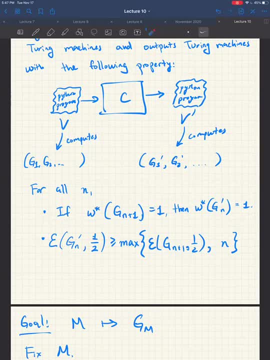 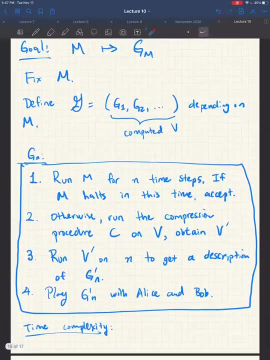 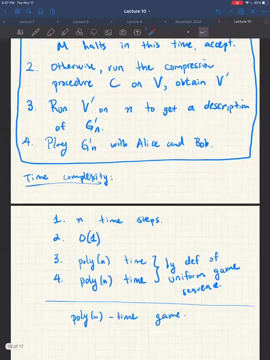 the max of the two? Oh, OK, I'm going to ask you after the class. Sure, Yeah, I think maybe it'll be more helpful if we see how it's used. OK, So we're going to. so I've just defined some game and now let's start to analyze it. 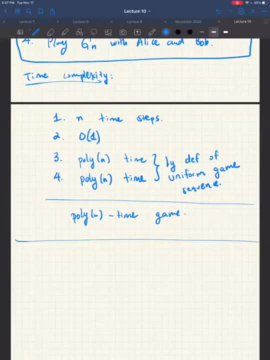 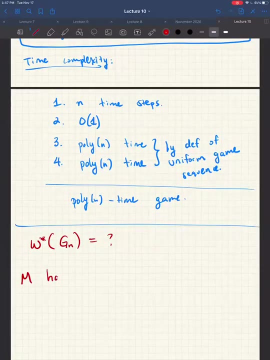 some sequence of games. So you want to analyze omega star of gn, Yeah, Yeah, Yeah. So let's consider two cases. Let's suppose that this Turing machine halts at some time, So say it halts in time, t. OK, then, for all n that's greater than t, and I think Yuval. 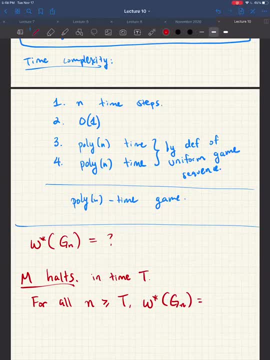 was alluding to this. by the way we've constructed this game, the verifier will have enough time to run this program out to completion, right? So the program is going to complete and then the verifier is going to accept. and Alice and Bob aren't even involved in the game. 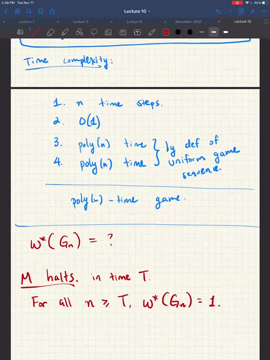 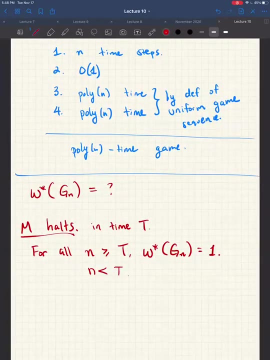 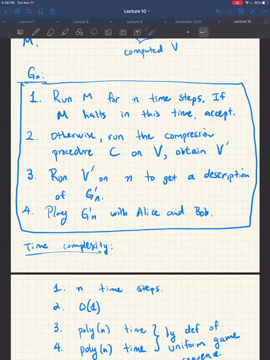 So the value of this is 1 by construction, right? Hopefully that's clear. So what about n less than t? Well, let's look at, let's just think about the pseudocode. So this step one will never terminate, right? 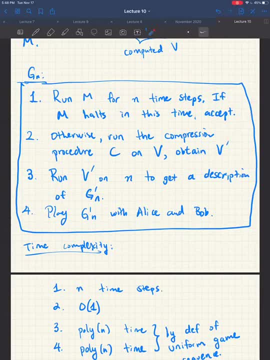 So we're just going to automatically move on to step two. We're going to run this compression theorem procedure, We're going to get a description of this game g prime n and we're going to play this game. So this game gn has effectively become the exact same game. 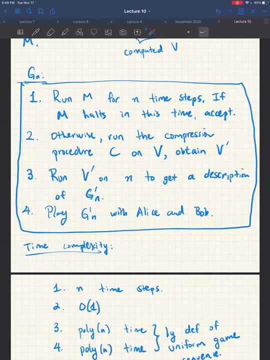 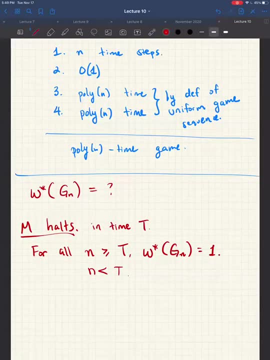 As g prime n, because you're just following all the same rules. So in this case, game gn is, you know, equivalent to g prime n by construction. In particular, they must have the same optimal winning probability, And what we're going to do is also add the winning probabilities. 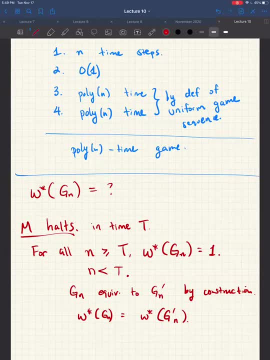 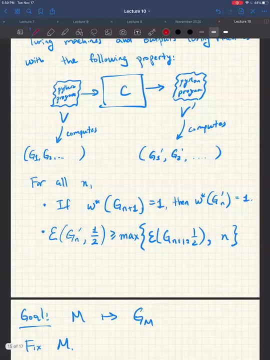 Okay, But what do we know about the winning probability of g prime n? Do you remember from the compression theorem? there You all were about to say something Who? Yeah, I think you had it earlier. so, Oh, yeah, like it will be one if the value of the 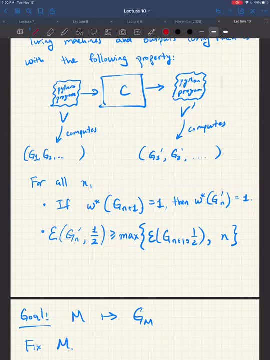 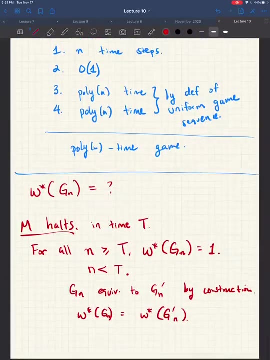 prior game in the original sequence was one, but you will just do that again, and again, and again and again until you reach T, and then it will be one. Exactly so you can, you know, so we know, that you know. so we have a kind of like an anchor. 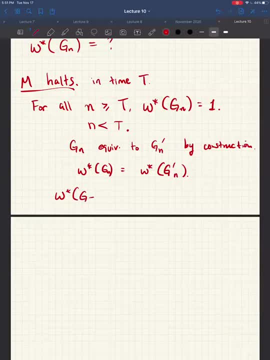 that Omega star GT is equal to one is equal to one, but by the compression theorem that must mean that G prime of T minus one is equal to one, Right. so those are by the compression theorem, And then we just kind of like ricochet down for all in. 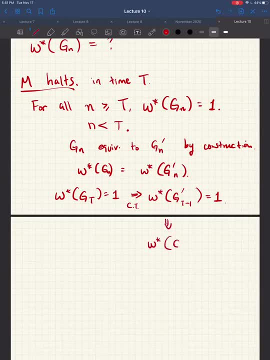 Right, and so that implies Omega star of GT minus one, without the one, is equal to one, And then, you know, we just sort of carry out this game BN�� Right, and so we just deduced that for all n. 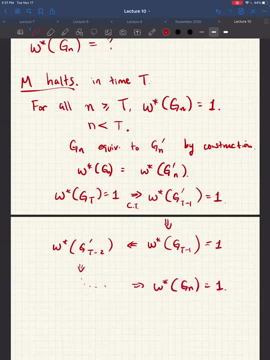 this game must have value one right. This comes from the using the compression theorem over and over again. Okay, so maybe this is the thing I'm not seeing. Why does the second arrow hold, Like the one that goes down This one? 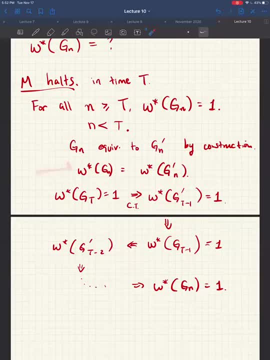 Yes, Oh, this comes from this statement. So this comes from this equivalency. Yeah, yeah, yeah, yeah, sure, sure, thank you. Can you say again why that statement is true, Because I'm missing that point. Why are the games equivalent? 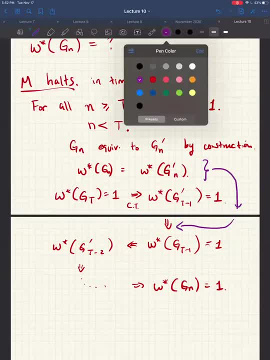 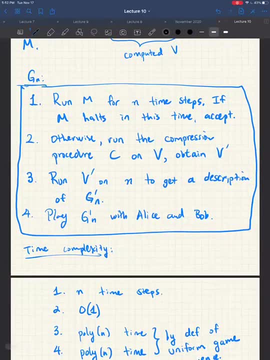 Oh, they're equivalent because you know we're asking: what is the maximum success probability of Alice and Bob in this game? It only depends on the questions and answers, like the decision rules and the sampling of the game right, And what game is being played with them. 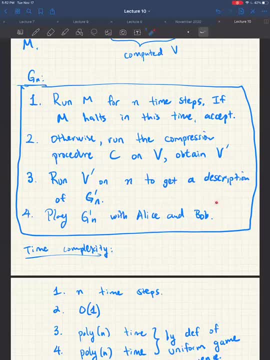 it's this G prime n like this is all that really happens, in some sense Like steps one, two and three are all just like happening behind the scenes in the verifier's head. Wait, but okay, so instead of step one, if we accept, then it's over, right. 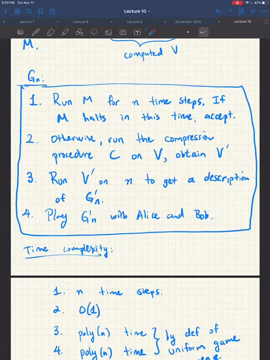 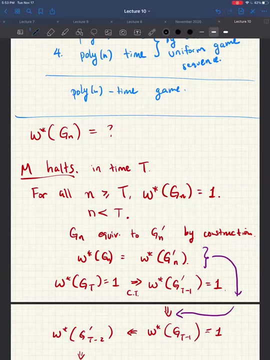 So if omega star of Gt would be one, but Gt never plays G n prime, So wouldn't that not be equal by construction then? Oh yeah, I was this: by constructions we're considering n less than t, So assume n less than t. 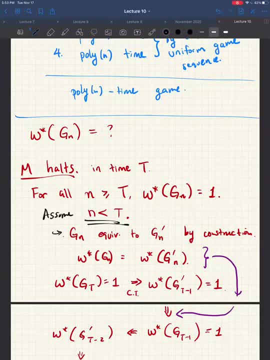 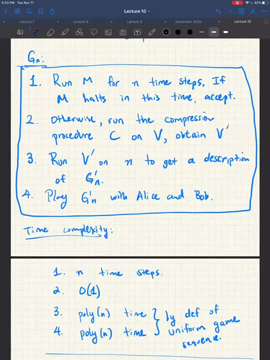 then, then then we have this equivalent. We'll go and see So. so like say n is less than t, then step one, like you can just imagine, like you always just pass over it. Okay, okay, okay. 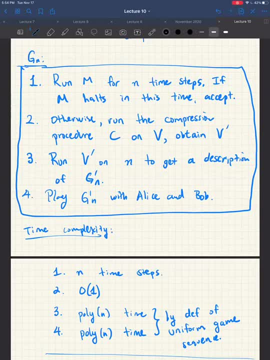 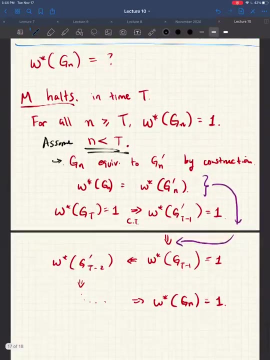 Ariel. does it make sense now? Yes, I think so. So there are a couple of points I need to think more about, but I don't have like questions, Okay. so it's sort of. by the way we've set up this game. 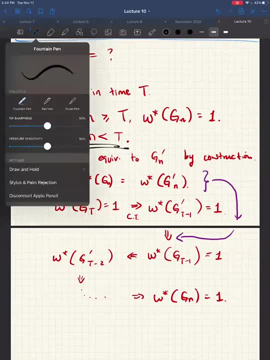 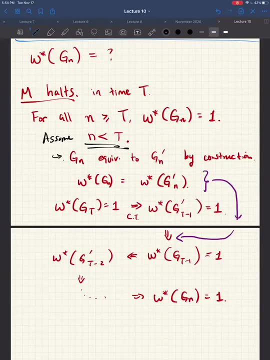 That's why we have this equivalency. Yeah, the earlier question I asked, that I'm clear on. Okay, cool, great. So the second condition you need for sound: there is a function, right? So the second condition you need for sound, 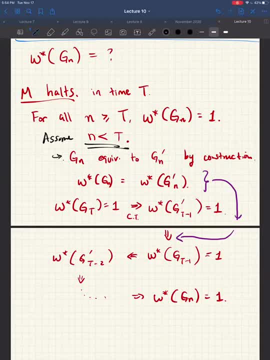 Yes, So right, So we're done with the M. like, if M halts in time T, then we, you know, in any time. then we know all of the games in this original sequence: G1 up to G2, G3. 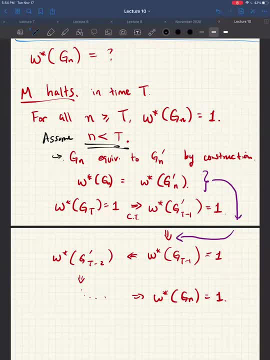 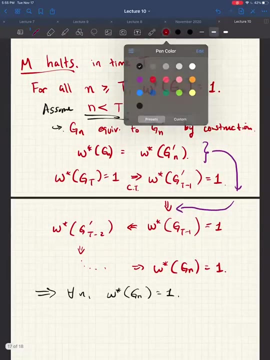 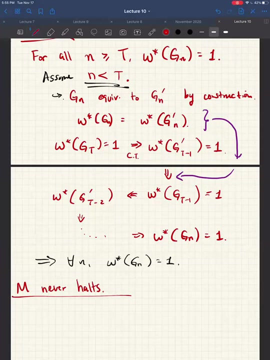 and so on. they all have value one, Okay, So we're at least good on that front. and the halting case. What about the non-halting case? And this is where this entanglement lower bound comes in. So suppose that it never halts, right? What's going on? So, again we. 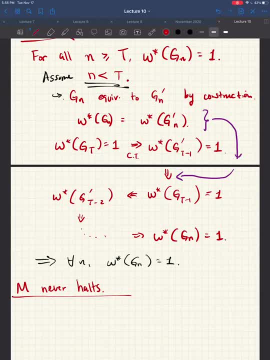 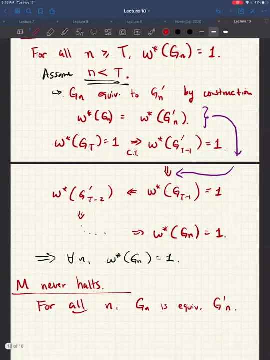 have this equivalency between GN and G prime N. So for all N, you know these two are equivalent games by construction And it looks like you've all had a flash of realization And but you know you say, well, okay, well, let's. 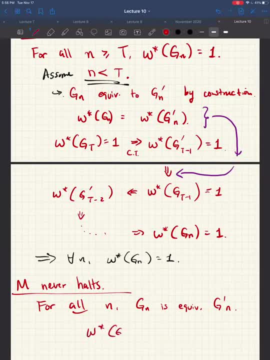 think about you know Omega, like we really want to show what Omega star GN is, but how do we relate it to? You know, okay. So so we, we know that, we know that you know this is true like. 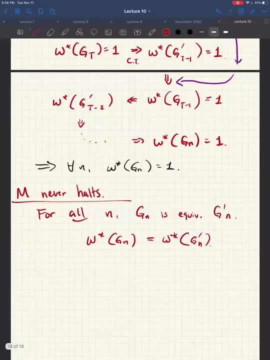 just by the same reason, But what we can't really do anything with a statement because we can't relate this to. I mean, we we know by the compression theorem it's related to GN plus one, but then what's GN plus one? And like we're kind of like stuck in circles. 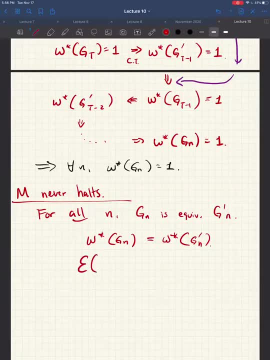 But this is where we use this entanglement lower bound. We also know that these two must be equal right Because they're the same game. But the compression theorem tells us something about G prime N. It says that whatever entanglement you need, it has. 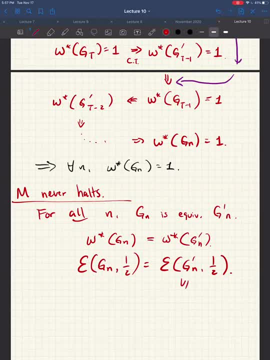 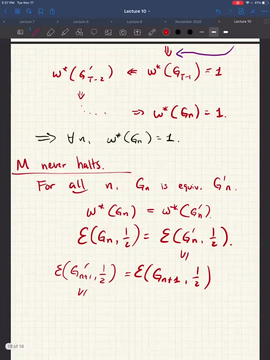 to be at least the entanglement you need to play the N plus first game in the original sequence. But since GN plus one is equal to G? N plus one prime, these have the same entanglement requirements And this is bigger than GN plus two. 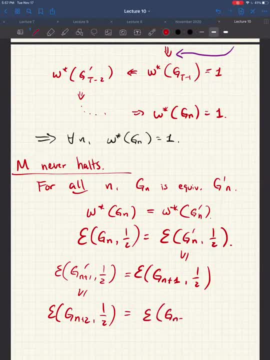 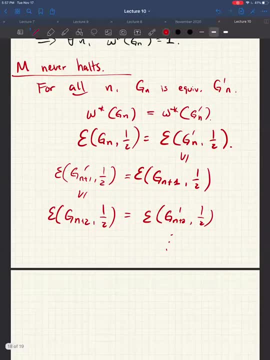 Right, And maybe you can see where this is going. Okay, So we, we have to. we have, like, this infinite chain of greater thans. So what do we conclude? That, whatever entanglement, you need to play this g? nth game. 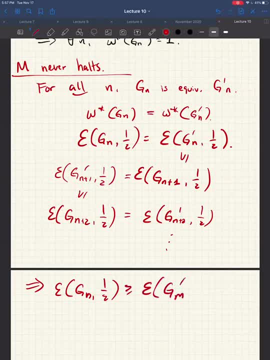 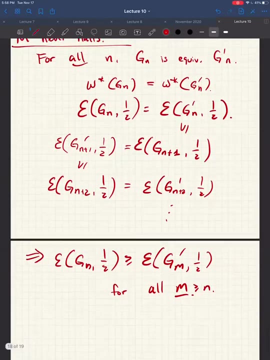 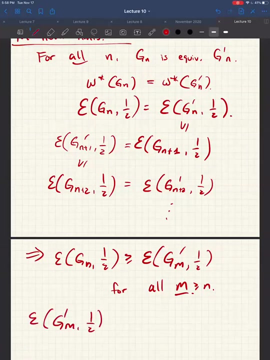 this has to be greater than g m prime for all m. Okay, But remember that this entanglement lower bound gave us a max, And we also know that g m prime has an entanglement lower bound of m. So you put the two together. 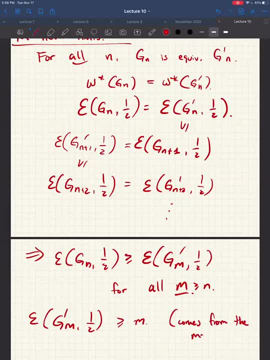 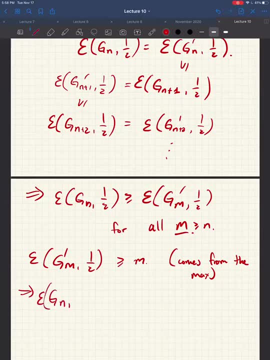 So this comes from the max. So you put the two together and this implies that entanglement of g n to win, with probability a half, is greater than m for any m you choose, Right? So there's no finite lower bound on this entanglement. 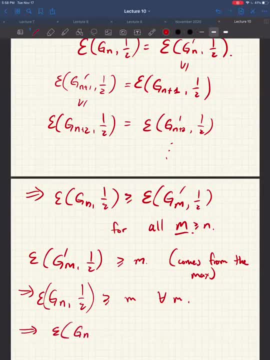 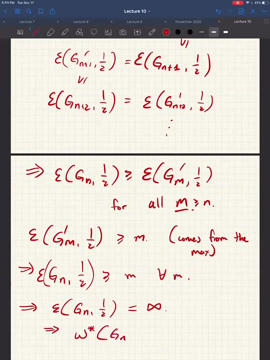 Right. So this implies that the entanglement needed to play this game, with probability half, is infinite, And it tells you that there is no finite dimensional strategy that can do better than one half. What does that mean? We can actually deduce something about this optimal. 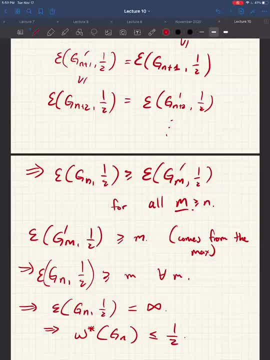 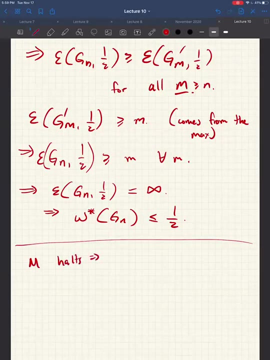 winning probability, It has to be at most a half. Okay, So we're basically done. We've shown that if m halts- and for any n, this is one- if m never halts, then this is at most a half. 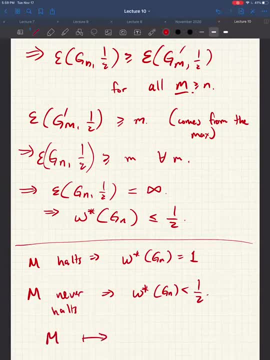 And so we can complete our reduction by saying that someone walks up to you with a Turing machine m you can just produce the first game of the sequence and it'll have the properties that you want, And so that completes this. this MIP star equals RE conclusion. 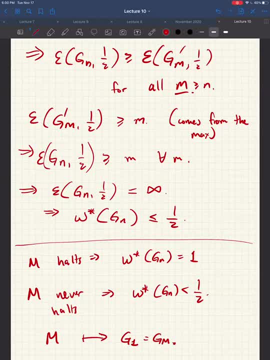 Well, you did not show us how the compression works. Yes, that's, that'll be for next time, But, but, assuming compression, we can do this basically recursive self compression, And this is how we encode whether a Turing machine halts. 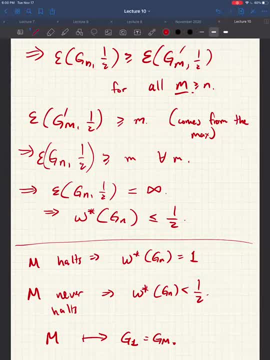 or not in a normal game, And it's six o'clock on the nose. Yeah, next time we'll. we'll see how you prove this compression theorem. Wait, sorry, maybe I missed it. So what is the precise connection between the complexity class, MIP, star? 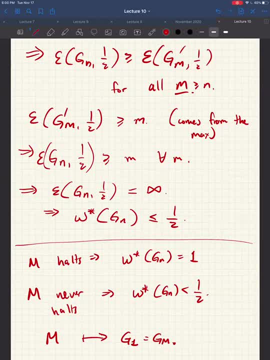 and the problem of approximating omega star. It's complete or like. did you mention this? No, I think I glossed over it. Yeah, basically it's a complete problem for MIP star, And why is that Good question? 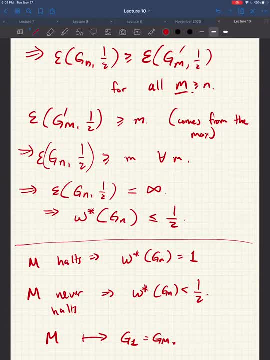 Well, I guess there's different answers to this. Okay, so the first answer is that approximating the value of a non-local game is constant. It's not text. And then the second, prior was: what is consistent Automaticallyiles is linear. 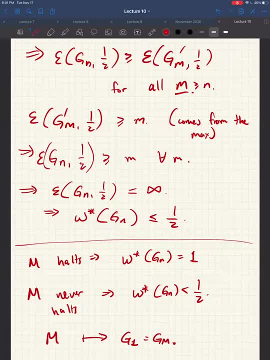 but the first one is invariable, Then挺ickers is linear, And the third way for 뭐야 is the services that all I attempt sort of stitching together, But it's sort of different. Yeah, I mean, that's kind of like I don't know. but I don't know pretty well what that is, Because there are different events or patterns between the. you know what all the competition individual analyzes is awarded against what sort of application is given. But you can. you knowjskett and others are programs And so you can be able. it'sちゃんllinger and justد Wuhan. 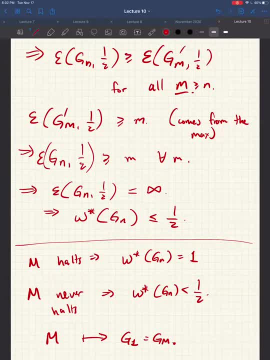 transform that into a non-local game with just two provers. uh, oh, no, sorry, with uh, it was just one round of communication. oh okay, yeah, wait. so which is the? which one is the strategy that you follow? so it's the one that you describe here, i mean in your proof. yeah, and they also describe: 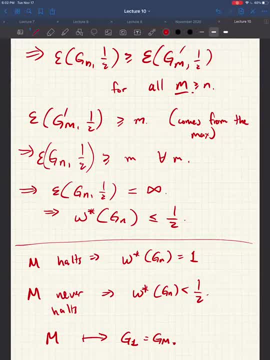 the other way of doing it. oh, the other way of doing it, it's that way. just shows that the the game problem is complete for mip star, but it doesn't show a lower bound. yeah, but i i won't be talking about that. even if the mip star protocol has a number of uh of communication rounds, that depends on n you can. 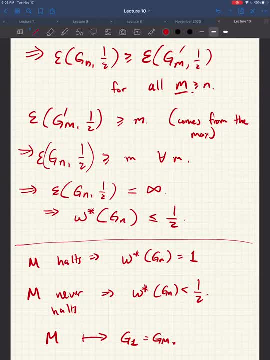 still reduce it to just like one, two and that's it. wow, okay, yeah, it uses, um, actually a lot of the stuff you've seen in this class, like rigidity and the hamiltonian problem and so on. who proved this round reduction result? um, uh, the first, uh, yeah, the first paper to prove is by uh jeng feng ji. uh, and then, and then we had a. 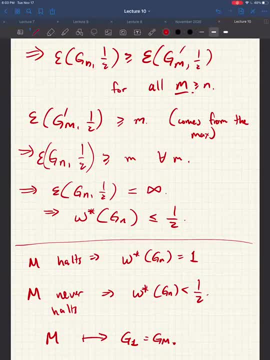 follow-up paper, that kind of uh. yeah, simplified it a lot, but i think, yeah, jeng feng was the first to to prove this. i guess the issue with that, though, is um. in this round, reduction increases the number of provers. i mean by constant number, but it's still uh, you know you don't get it for. 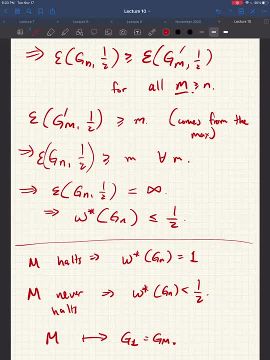 free. is this also true for q ip? that, that is, that, like each, you can just reduce it to one, two, yeah, and that's it. and this is not known to hold class. classically, right, um, classically, uh, it is true that, uh, all mip protocols are convertible to um. 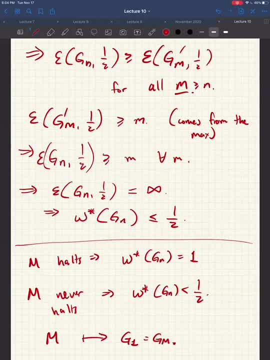 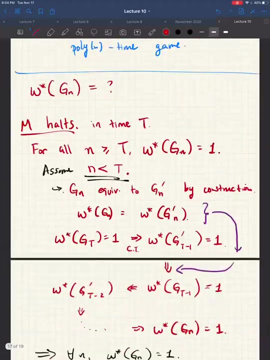 you know two proof or one round- uh, this is also known. or all mip protocols- yeah, but not all ip protocols. that we don't think is possible. i have another question about the halting problem. yeah, i'm wondering, because b has a problem with that, this sort of property that, uh like, if b halts, then b goes into an infinite loop and vice versa. 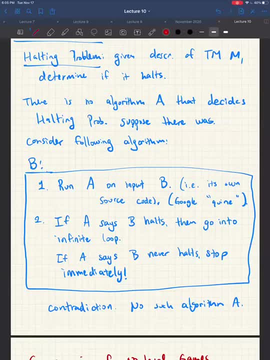 i'm wondering if you make like a promise to only include like algorithms that don't have this sort of contradiction in them, so like like b halts, if, and only if, it doesn't go in an infinite loop, then would there be something that could tell you an algorithm holding algorithm? 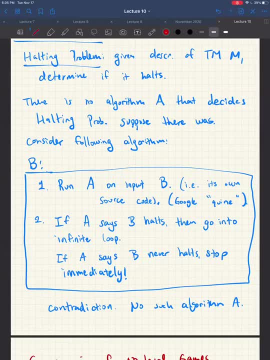 i think the tricky part there is like formalizing what it means for an algorithm not to do something tricky like that. um, i think it's just really, really hard to get around this style of halting contradiction. um, okay, so uh, if i remember, there's something called rice's theorem which shows that. 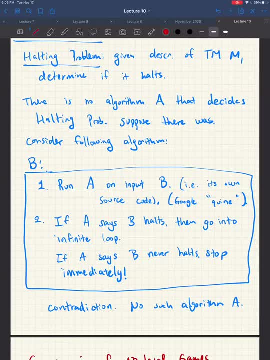 um, anyways, you can google rice's theorem and i think it's might answer your your question. it sort of says that: uh, it kind of says, yeah, you can try to institute all sorts of different properties, but a lot of them will end up being undecidable. um, maybe someone who's taken a computability class more recently can say more. 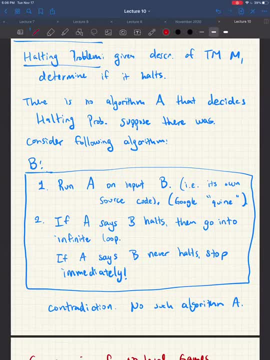 like in general, most properties are are indecisive and they're not indecisive and they're not compatible. yeah, i guess my sort of intuition about this and i i haven't taken any course like this, but my intuition is like we humans can, like, look at these problems and figure out when, like it would not be. 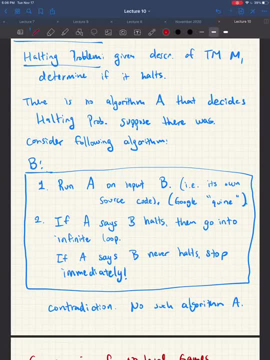 able to like. it doesn't have either a halt or not halt, so like there's some algorithm running in our brains, right, but maybe there's ones that we couldn't even figure out before. yeah, um, i mean, i think you know not to put down our own brains, but i think we just haven't looked. 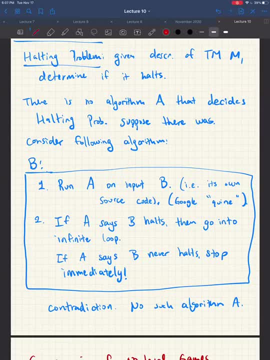 at that many actually, you know. but if you've divided any program you can, it can be really hard to figure out if something halts or not. um, i i would say, uh, just like on that point, um, i don't like his ideas, like i would say i disagree with what he says. but roger penrose, um, actually says, 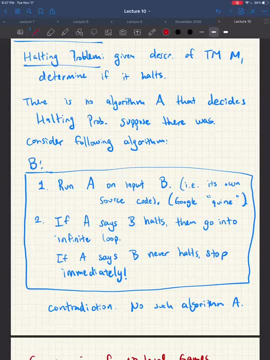 like the human mind is uh like exactly in line with the idea of the universe, uh. but i think it's like the human mind is uh like exactly in line with the idea of the universe, uh, but i think it's way capable of you know mathematical insight and can see the solutions to things that 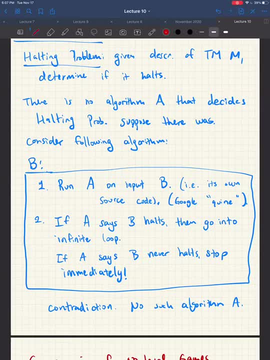 are uncomputable, um, and he has like his theory of he, he had whatever he, he wrote like books about this one which i read um, which i don't find convincing, but like he argues, he does argue that and you know, like roger penrose deserves consideration, i guess. cool yeah. 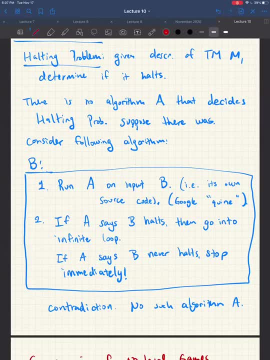 i think, um, it's, it's definitely worth, yeah, it's a argument worth considering, um, but i think, uh, you know, even in in practice, you know i don't know how much software debugging roger penrose has tried doing, but i think you know, general can be quite difficult. so at least from experience i 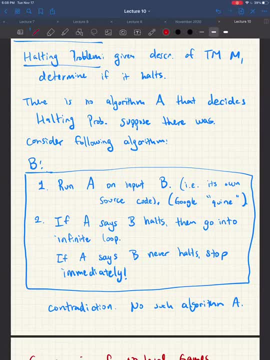 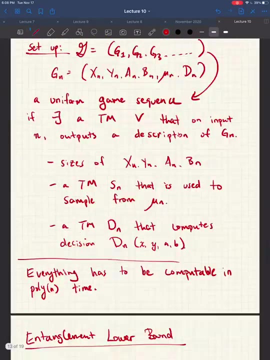 believe the halting problem is unsolvable. um, i have a very uh basic question about the definition of compression, so i'd asked you earlier in the lecture. this was the? um, the entanglement, uh property, there, uh the entire step. so you have a max there, uh, and 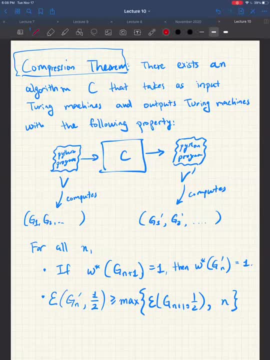 the choice of the uh cap of n. is there any specific reason why it's n, um and uh, oh, you mean, you mean this thing here, yes, oh, uh. so it doesn't really matter what this is, it just needs to be a growing function, like we never used the fact that it was n per se, but it just sort of goes off to infinity with n. 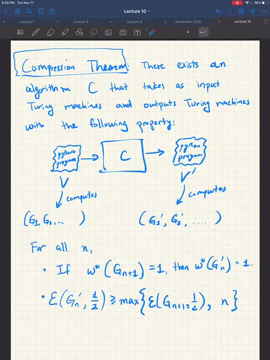 okay, yeah, that's what i was asking about. okay, so i guess there's no worries about you know being having a large enough cap uh in relation to your choice of the, the input g uh of m plus one uh and its entitlement value, like um, its relationship to 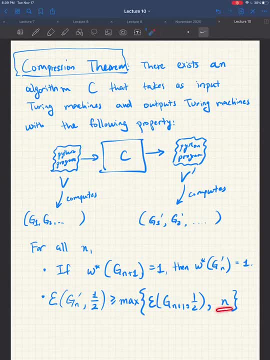 the choice event. yeah, it's not so important. i mean anything that goes infinity, uh would make the argument work okay, and uh, just a point. other question i'd mentioned was about the that uh some guy in waterloo here had uh done a presentation on this. uh c? uh the cep, uh problem parliament. uh he was. 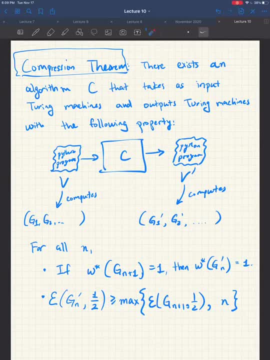 talking about some uh, uh, for these non-local games, that you can have this affiliated uh, c sharp, sorry, c- star algebras, and that the, the representation theory, can tell you if the game has a perfect strategy or not. um, for each of the possible models, um, and i was just wondering, uh, if that is of any. 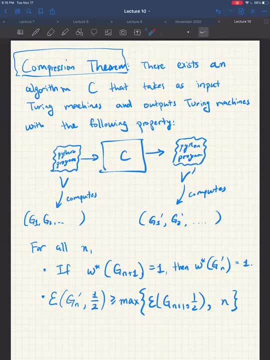 interest with relation to uh cep as an algorithm for uh determining these, uh, the, the, uh, so the winning probability or the optimal strategy. oh, i see, oh, i guess. yeah, i mistook what you said earlier about c-sharp. i thought you were making a joke about that. i meant c star. 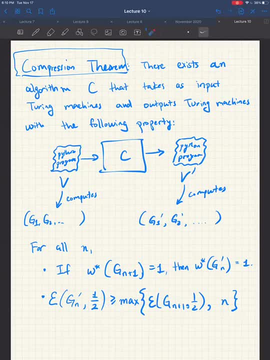 i saw some guy called von paul paulson, i think, from university. yeah, there's a presentation on that. yeah, um, i, yeah, i, you know, uh, i guess you know that's sort of like a whole another thing to get into, but um, definitely, yeah, there's um, um, one of the questions that's. 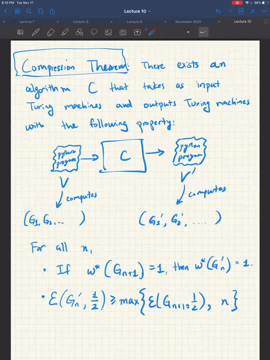 that remains open from this uncomputability result is: uh, you know how can we actually get a handle of the algorithm and how can we get a handle on it? or on describing what this, you know, infinite dimensional community operator strategy that supposedly does well, um, uh, you know what does. 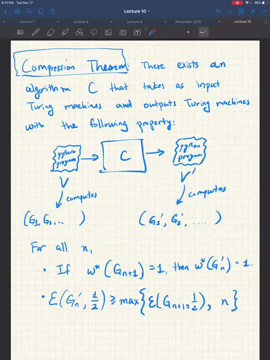 it look like you know can. can we describe it? and this is something that you know, the math people are very interested these days. um, like we know it exists, but, uh, you know what are its properties? and um, the c star algebra thing that you're mentioning, i think, is a possible way to try to. 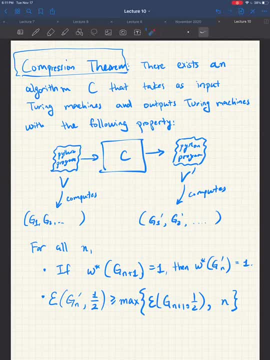 get a handle on it, but people are trying to figure this out, okay, thanks. uh, randy, you're very faint. i don't know if it's like your microphone or something. is that me or? uh? no, i think randy was trying to say something. uh, okay, maybe not. 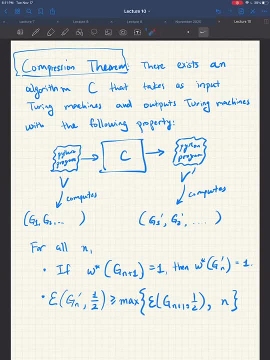 oh, okay, so you're typing, typing it right? yeah, so von eumann, algebra is our type of c star algebra, um, all right, so so, uh, you know, next week we'll dive in and see how you compress non-local games into algebra. so we'll see how you compress non-local games into algebra. so we'll see how you compress.